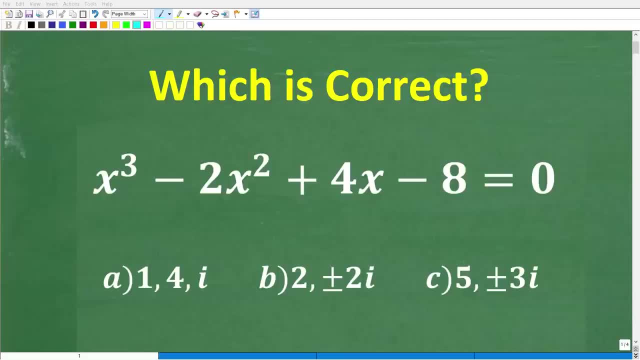 Okay, so let's see how much you actually know about solving polynomial equations. This is a tremendously important topic in algebra, And let's take a look at our problem. We have x cubed minus 2x. squared plus 4x minus 8 is equal to 0.. We are trying to solve for x, And this is a. 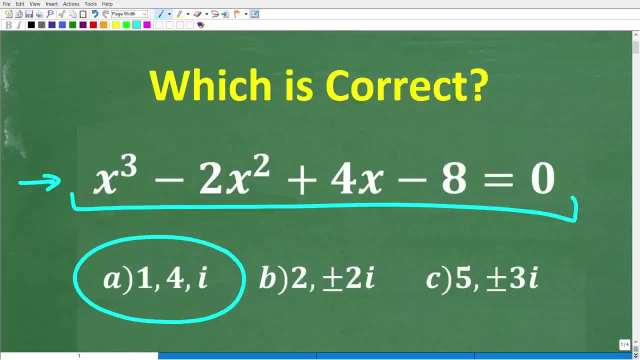 multiple choice question. So our answers are A: 1,, 4, and I B, 2,, plus or minus 2i, or C: 5, and plus or minus 3i. Now some of you might be saying, hey, Mr YouTube Math Man, I'm really. 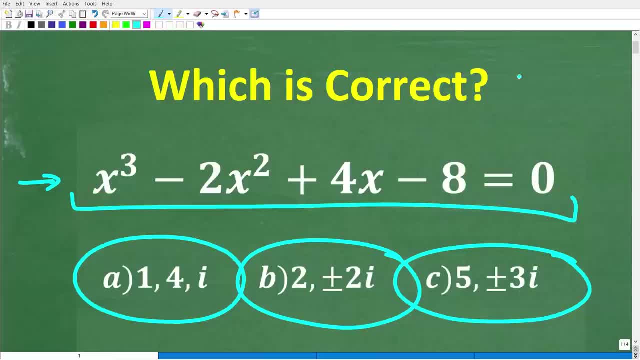 good at solving equations. Well, there's a big difference here in terms of solving equations- polynomial equations- because something as simple as 2x minus 1 is equal to 9,, for example, is a multiple choice question. So our answers are A, 1,, 4, and I, B, 2, plus or minus, 2i or C. 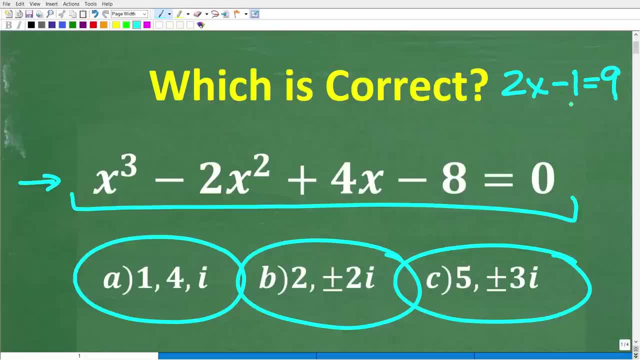 a basic polynomial equation. This is what we call a linear equation, and it's to the first power. So this equation is very easy to solve. Matter of fact, if we turn this x into a power of 2, made it a second degree polynomial equation, 2x squared minus 1 is equal to 9,. 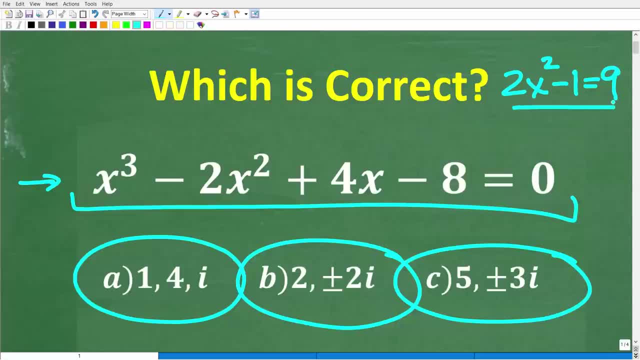 this is pretty easy to solve as well. What we're dealing with here is a quadratic equation, So some of you might be saying, hey, Mr YouTube Math Man. well, what's the big deal here? This is easy. This is x to the second power. But over here we're jumping up one power from x to the. 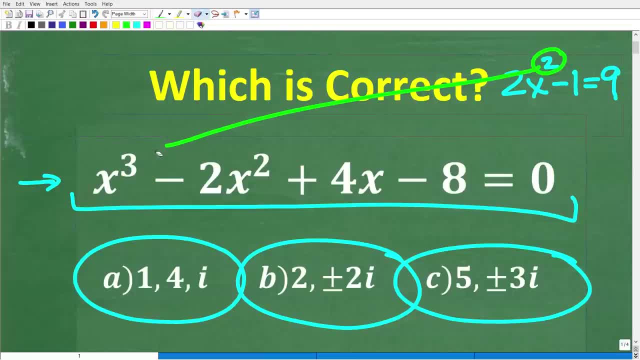 second power to the highest power, here being 3.. Well, when you go from a second power- polynomial- to a third power polynomial or higher, things get very interesting pretty quickly, And I'm going to cover everything that you need to be thinking about in order to solve these type of equations. 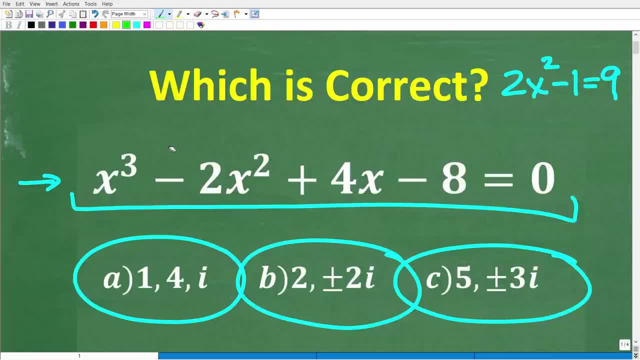 If you're taking any sort of math course like Algebra 2,, College Algebra, Intermediate Algebra, Pre-Calculus, this is something or this topic is tremendously important. You absolutely need to know a lot about polynomials And, of course, I'm going to cover everything that we need to really be thinking about in order to 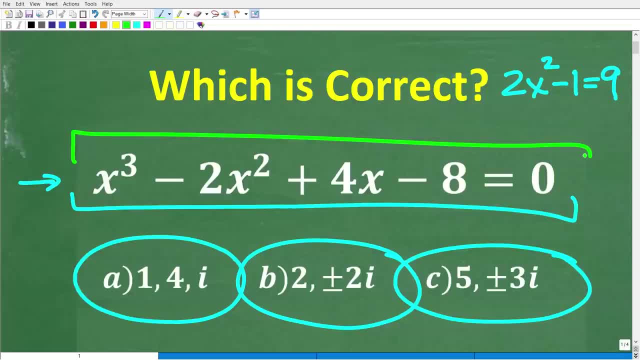 solve this problem. Okay, with all that being said, feel free to use a calculator, But if you can figure this out, go ahead and put your answer into the comment section. I'll share the correct answer in a second. Then, of course, I'm going to walk through exactly how to solve this problem. 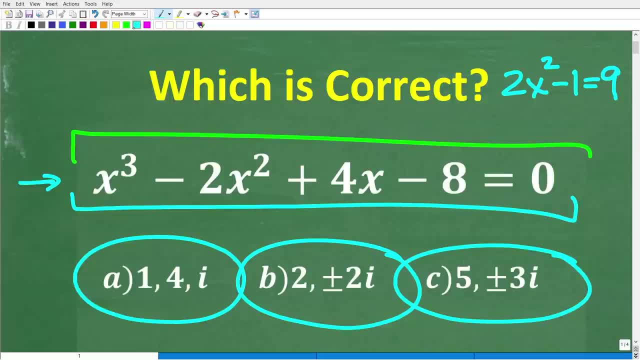 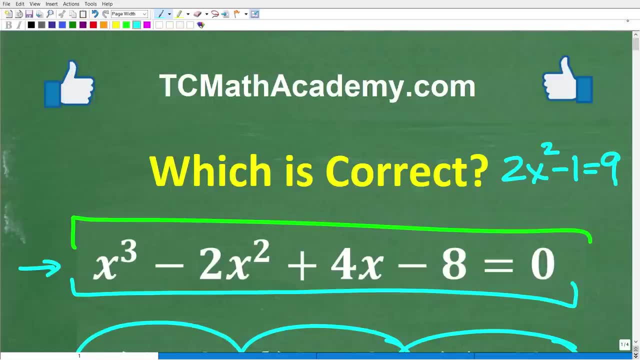 And I'm going to kind of do a quick review of all the things that you need to be thinking about when you face a polynomial equation. This is really important stuff. But before we get started, let me quickly introduce myself. My name is John and I have been teaching middle and high school. 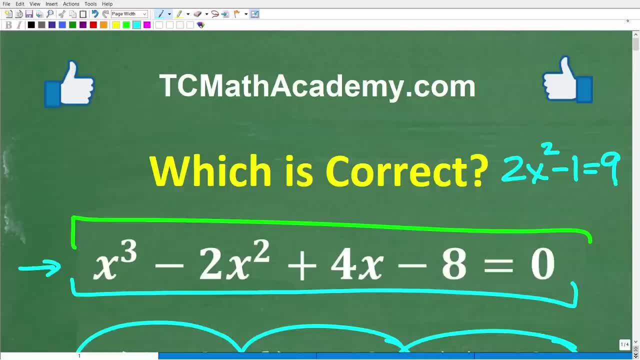 math for decades, And if you need help learning math, check out my math help program at tcmathacademycom. You can find a link to that in the description below, And if this video will help you out, or if you just enjoy this content, make sure to like and subscribe, as that definitely. 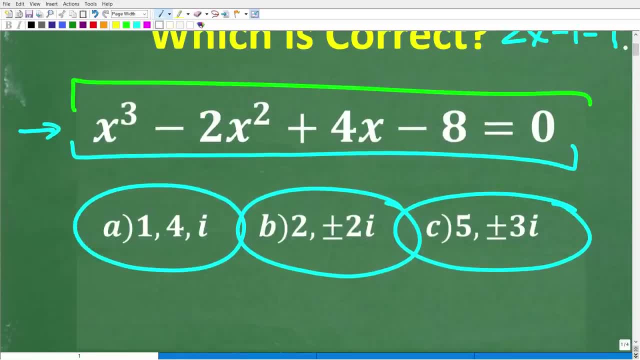 helps me out All right. so there's a lot of different approaches you can take here, And I am giving you the kind of really big advantage of using a calculator, right? So here is our equation. So x cubed minus 2x squared plus 4x minus 8 is equal to zero And the correct answer. 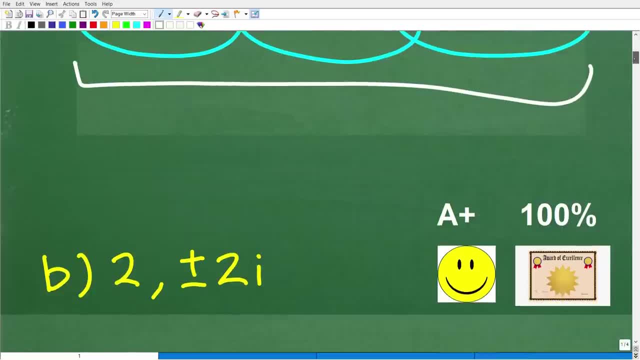 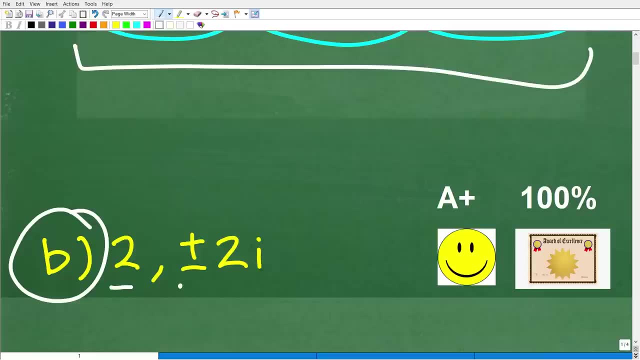 is one of these, And let's take a look at the right answer. The correct answer is b, So here are our solutions. We have 2 and then plus or minus 2i. Now I'm going to fully explain this. It's going to take a bit of work, But if you got this right, that is super impressive, Matter. 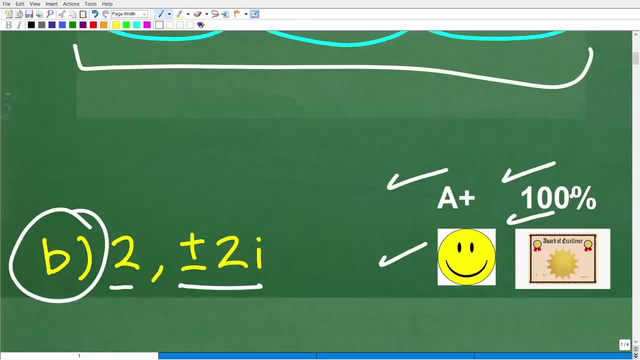 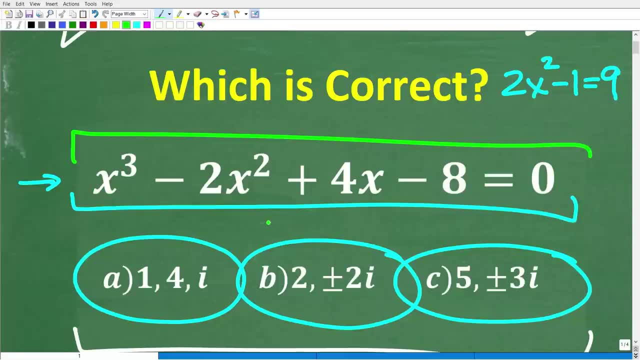 of fact, you definitely get a happy face, an A+, a 100% and a certificate of excellence, because you appear to be a certified professional expert in solving polynomial equations. Now you know, I like to kind of teach math in a non-classical way. I like to teach math in a non-classical way. 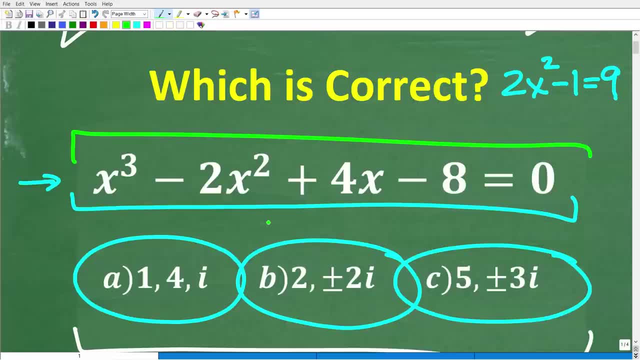 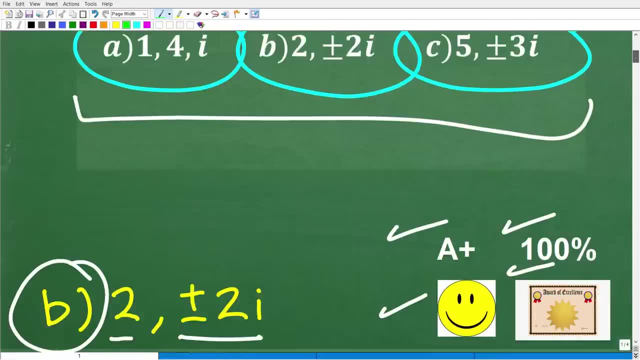 You know- and that's the great thing about teaching on YouTube- I could just kind of let my own personality shine through. So let's have fun with this problem. But we have a lot to cover, And the great thing about this particular problem is it is a multiple choice question. All right, 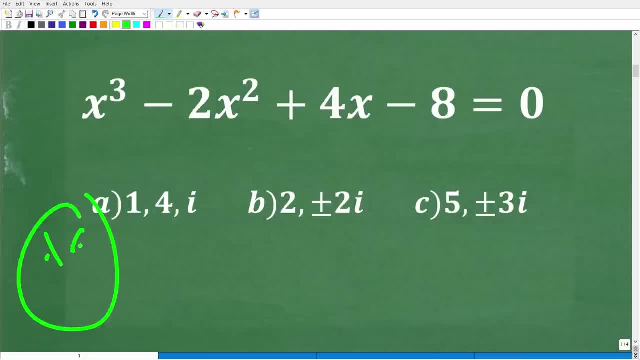 So some of you might be saying: hey, Mr YouTube, Math Man, I'm totally lost here. And what if I encountered this on a test? What could I do? Well, I suggest that you guess, right? So yes, indeed, I'm telling you. 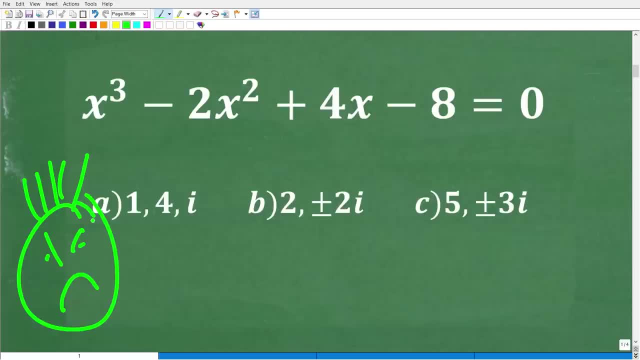 Take a guess. I mean, what do you have to lose? Now, some exams you actually do get penalized for getting a wrong answer, So you got to be very careful, But those are not too common. Matter of fact, tests like the SAT or ACT, you'll have to look at their policies, But typically you do lose. 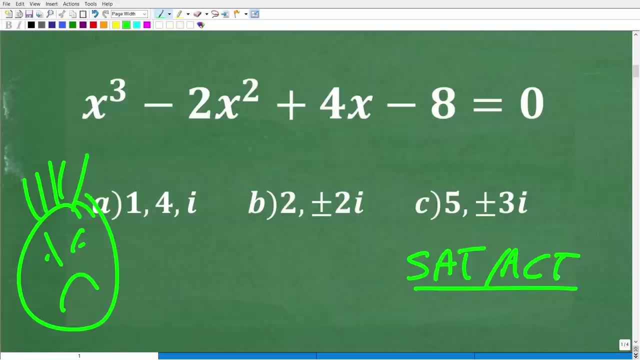 like a quarter point or an eighth of a point for wrong answers. But even so, in this particular case, you know, just take a guess, because most math teachers are not going to be able to get a right answer. So you're not going to penalize you for guessing right. But here, in this situation, 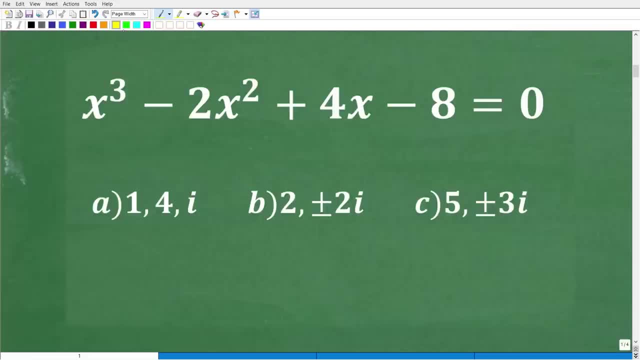 you can actually figure out the right answer if you know something about polynomial multiplication. right Now, here is what I'm talking about. So we know the correct answer is B. So what does this mean? Well, it means that we're solving for x. x is equal to 2. And x is equal to. 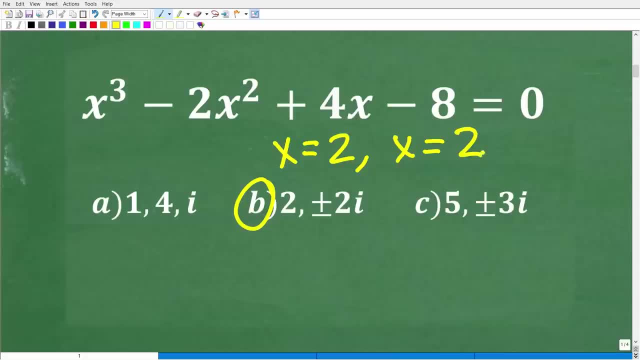 positive, negative 2i. So that means x is equal to 2i. And then we have, you know, x is also equal to a negative 2i. So when we have a positive 2i and a negative 2i, we just write it. 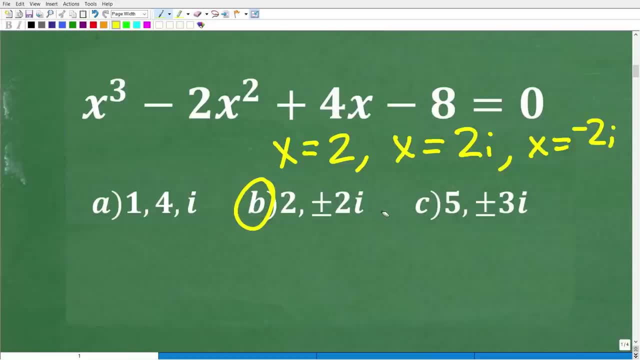 as positive negative 2i. Okay, so we have three solutions here. Now, if you can think of these right here as linear factors, all right. so what am I talking about? So let's suppose you have a basic quadratic equation and your answer is x is equal to 4 and x is equal to 3.. Okay, so this: 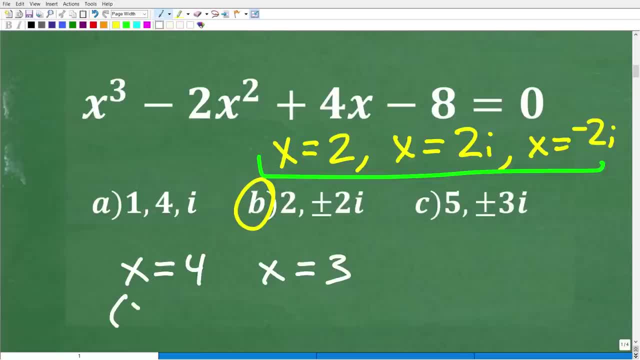 these solutions from a quadratic equation would come from these two factors: x minus 4 and x minus 3 is equal to 0. So I can kind of reconstruct the quadratic equation here, right? So if I had two linear factors, x minus 4 and x minus 3,? 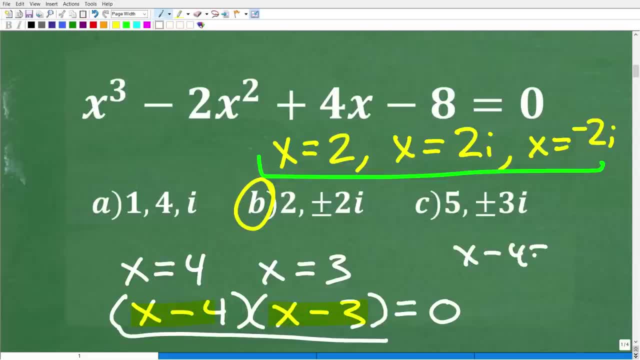 I would set each equal to 0, right. x minus 4 is equal to 0 and solve for x. So x is equal to 4, all right, So that would be one answer in this quadratic equation. Of course, we do the same thing with this other linear factor. So when you have 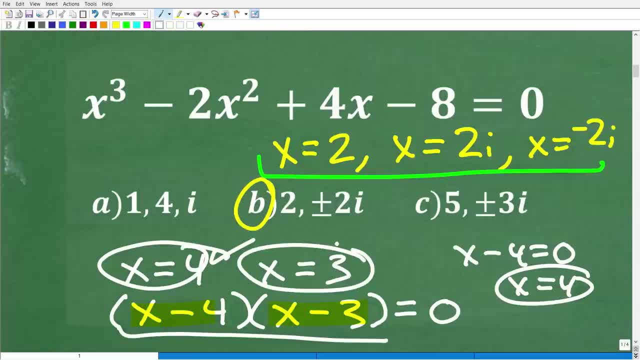 the solutions to a polynomial equation. you can just put those into linear factors and then just do all the multiplication and see what gets you back to the original equation. All right, so hopefully this makes sense And to understand what I'm saying here, everything I'm going to be 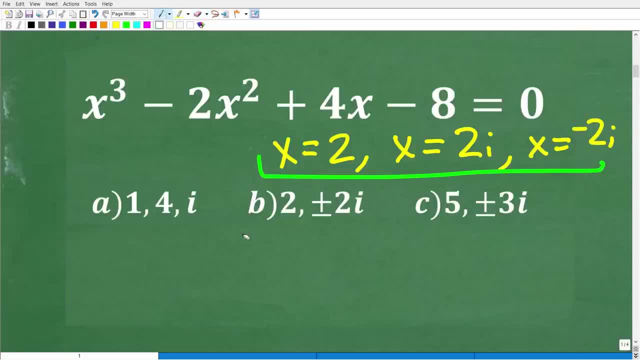 talking about, you need to be pretty, pretty familiar with solving quadratic equations And, of course, if you're not at this level of math, stick with me anyways, because you'll still be able to kind of learn this, even if it's for the 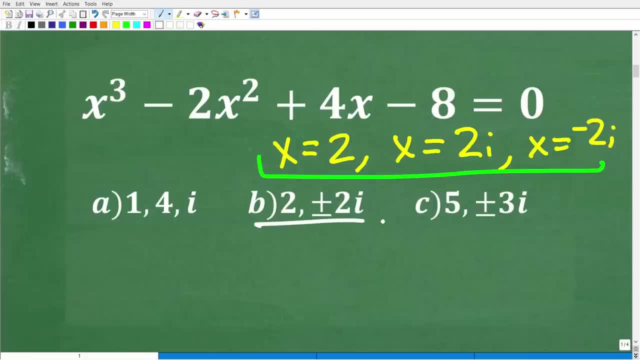 first time. All right, so here is our solutions. right? So we could be like: all right, x is equal to 2, so that came from the linear factor x minus 2, and then here 2i. I can write. I could go x. 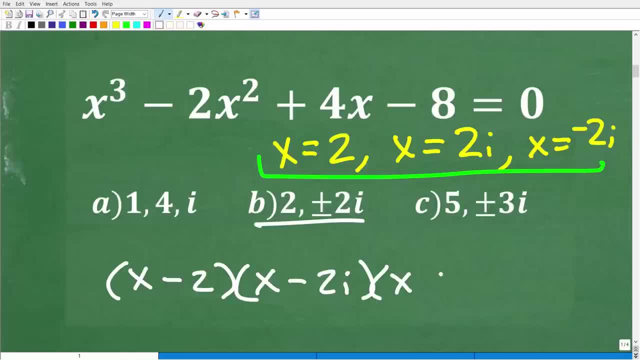 minus 2i and then go x minus a minus 2i. right here Now I'm not going to do all the work, but what you could do is actually do all this multiplication and it would get you back to the original equation. but that's a lot of work because you would have to actually test each one. 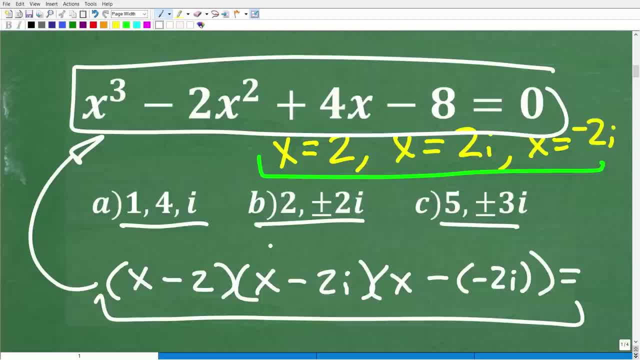 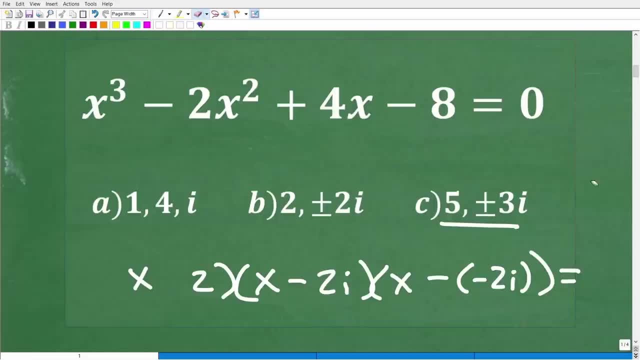 of those things, but another thing you could do, right? so this is one kind of approach. you could, and some of you are saying, hey, Mr YouTube, Math Man, you could do this as well. Indeed, you can. 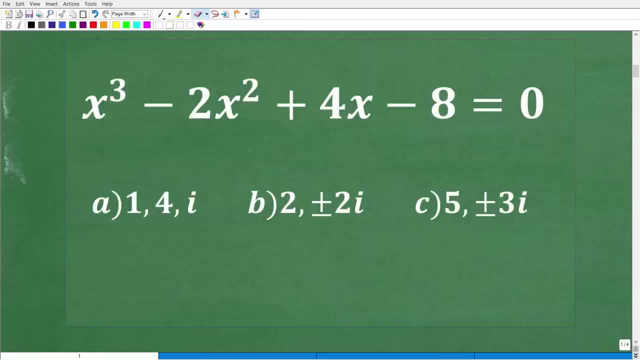 and if you're using your calculator, you have a lot of different ways you can, you know, figure this out. So if you look here, this equation has one right. I'm sorry this choice has one as a possible solution. 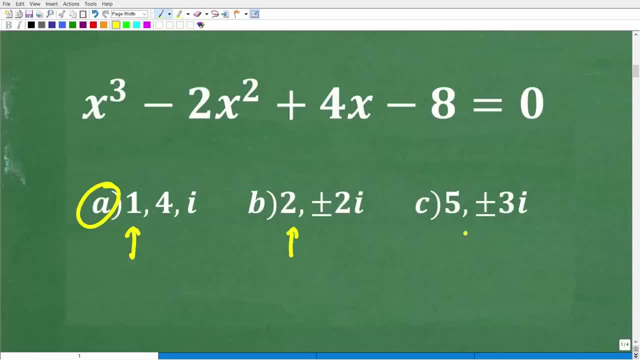 to our equation, right? so this one has two and this one has five. so we can kind of do a process of elimination by plugging in one for x, right? so some of you might be saying, hey, Mr YouTube Math. 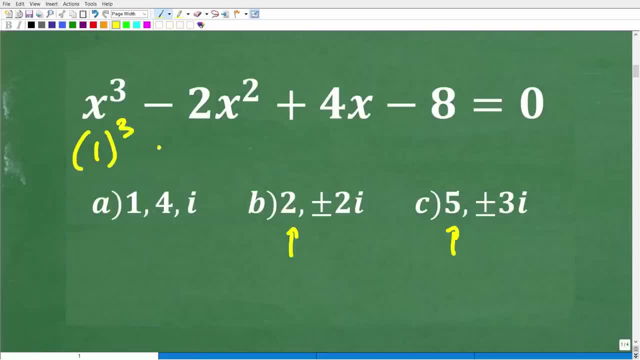 Man, that's easier. so if I go, one cubed I'll replace the x, and then I just kind of do this right: replace all the x's with one. this is not going to work out, all right, I could just tell. 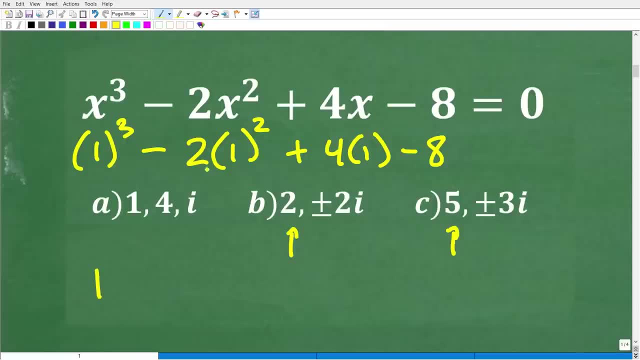 you right now. one cubed is what that is going to be. one minus two times one squared, so that's going to be one times two. so that's minus two plus four. right, four times one is four minus eight. well, is all this going to be equal to zero? Well, no, we're going to get negative one here. 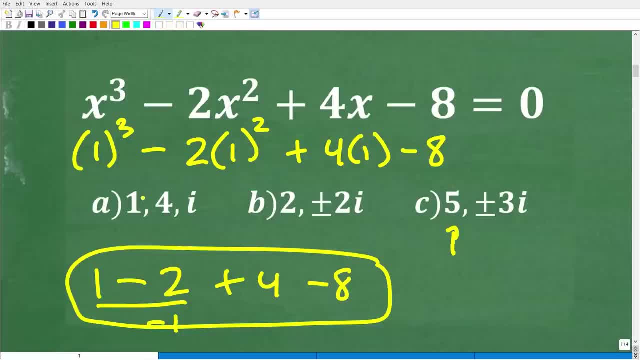 negative nine. so all this is not going to add up to zero. so one is not a solution. so this cannot be right. okay, now when you plug in two, you'll see that positive two is a solution. you just don't know about these things here. but if two is a solution, well, it doesn't show up in this answer. 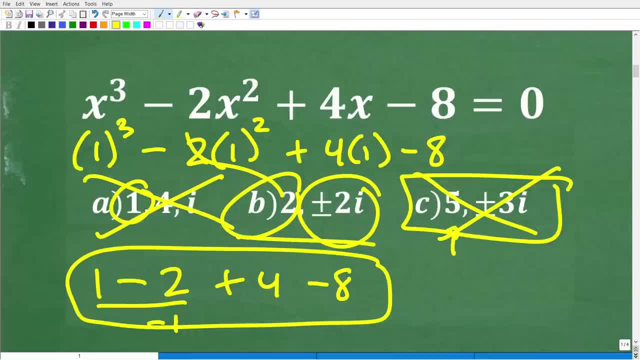 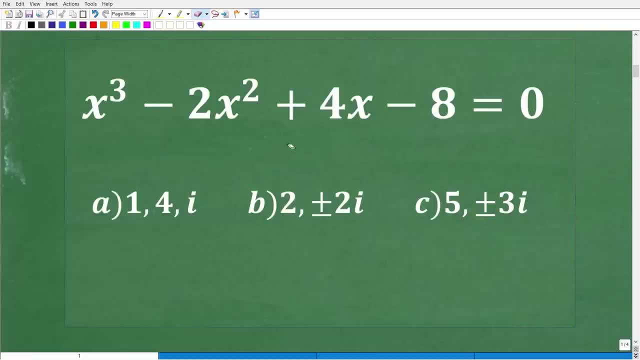 so b is correct as well. so there's really no excuses for you to get this wrong, and I want to fully cover this problem, because some of you that are taking, or are still students and have to take math tests, you know. I want to get you fully prepared so you can go in there and be like 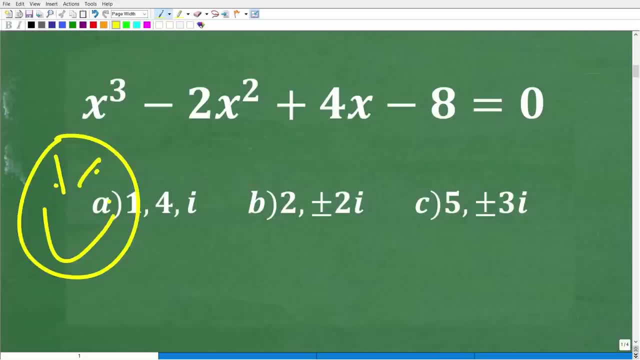 all right, Mr YouTube Math Man, I didn't really study, but hopefully you know for my exam. but hopefully I'm going to have some multiple choice questions on my math test and that is awesome. you know we'll put those in, but oftentimes they'll be like: no, I'm sorry, I just want to see. 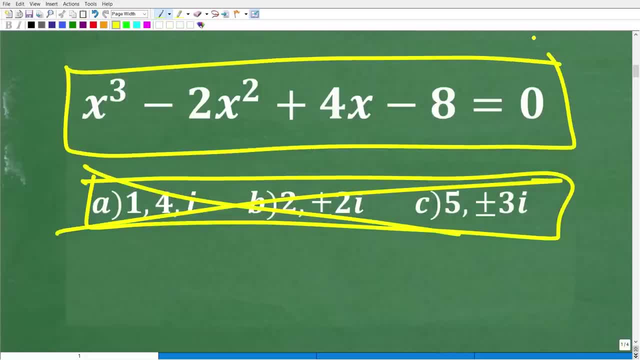 what you really know. so solve this thing, and you know, with no multiple choice options. so in this case, you're just simply just going to have to do the math, and that's what we're going to get into right now. okay, so here is our lovely equation. we are talking about polynomials, so I can say the: 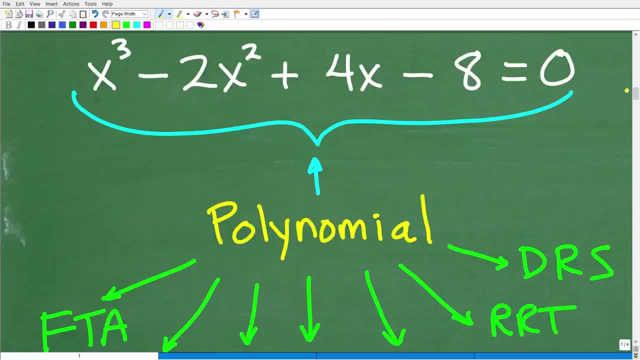 word polynomials, but I suspect three-fourths of the math students out there cannot define the what a polynomial is. now they might be saying, yeah, I know what a polynomial is, Mr YouTube Math Man. I see it all the you know, everywhere and all the time in my algebra course or math class. 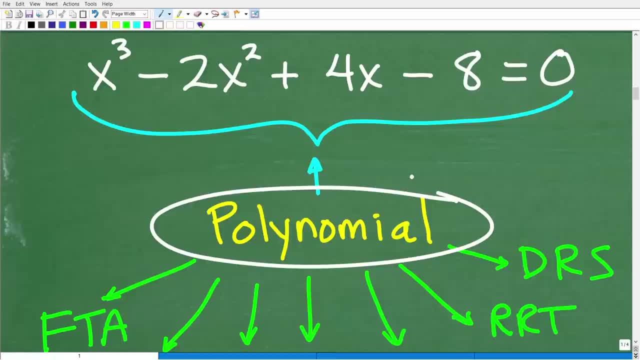 but what is a polynomial? Well, what we're dealing with here is a polynomial equation, because not everything in math or in algebra is a polynomial. so it's very, very important that you understand what a polynomial is. matter of fact, let me go up here real quick. 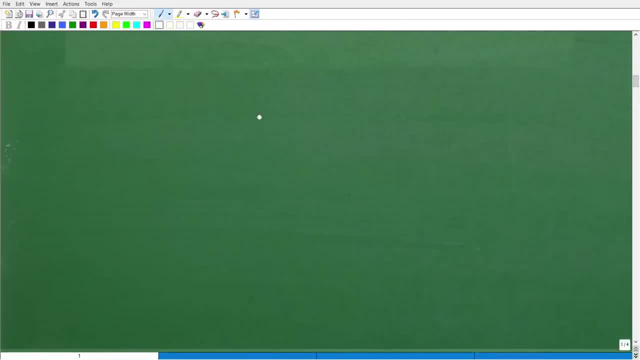 and just quickly define it in a rough kind of way. so let's just take a variable like x or y, it doesn't make a difference, you can actually have a combination of variables. we'll take a simple variable like x. now there's two parts to an algebraic term. 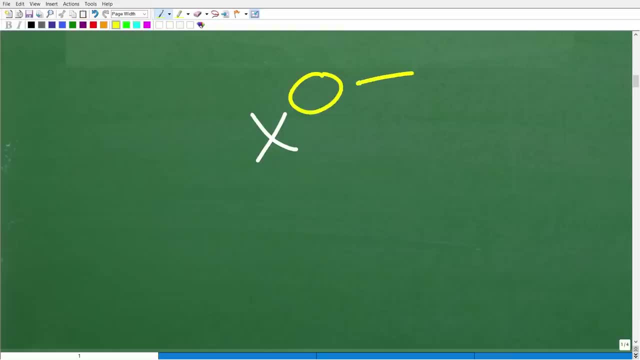 right now for us, we're going to consider powers right up here, okay, or the exponent to this particular variable, and then we'll consider coefficients, what we can put in front of the x, all right. so let's just kind of settle this right now. 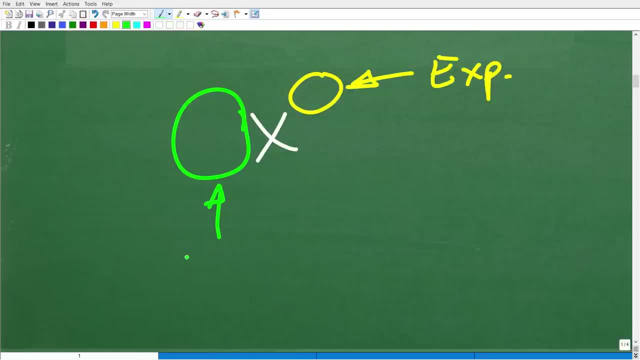 and we're talking about what a polynomial is here. right, we could put any real number we want in front of the x, and it's still a polynomial. so I could put three, or I could put negative 0.9, I could put pi, I could put two-thirds, so you can have any coefficient in front of the x. 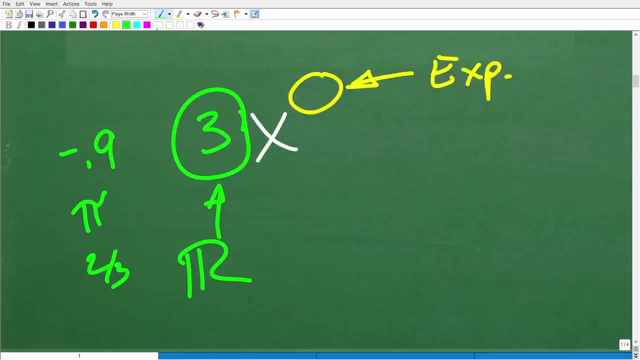 no problem there, all right. so the real thing to be very careful about what a polynomial is, is the power, the exponent. so the exponent to on a variable- okay, like here on a base- can only be a positive integer or a whole number. 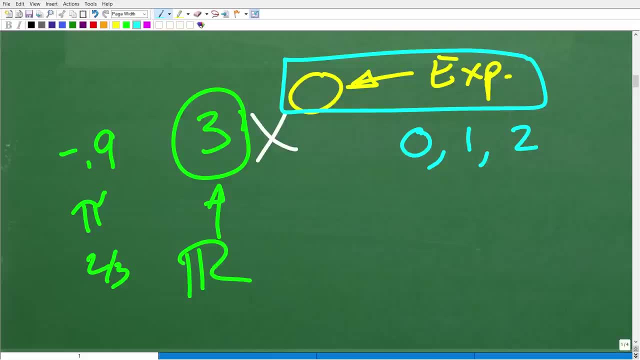 so we're talking like 0,, 1,, 2, etc. so if you have something like x to the one-half, this is not a polynomial. okay, this is not a polynomial. matter of fact, this is equal to the square root of x. we're talking about a radical equation, okay, so that's something. 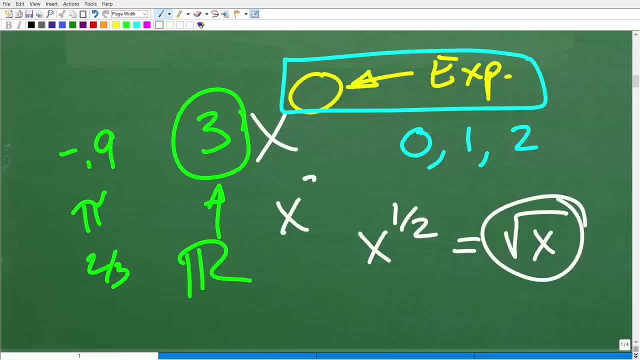 different than a polynomial. but if we have x to the, you know second power, that's a quadratic equation, that is a polynomial. now, it's important that you know the difference between the two, because I'm going to get into things that only apply to what a polynomial is. 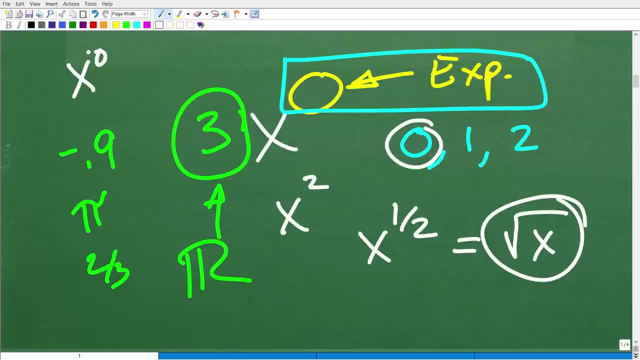 now, even x to the zero power is a polynomial. okay, so this is one term of a polynomial. we start stringing multiple terms together, then you have binomials, trinomials, etc. etc. okay, so I am covering a lot here, but just think, by the time I finish this video you're going to be 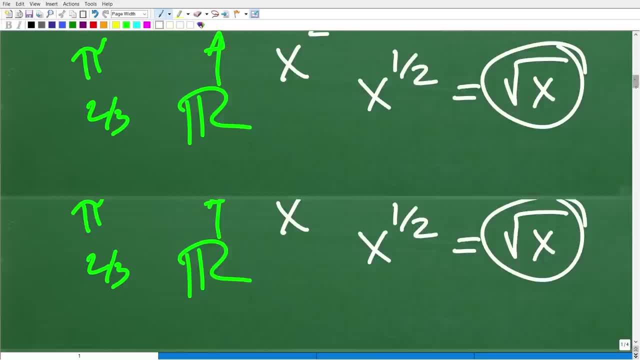 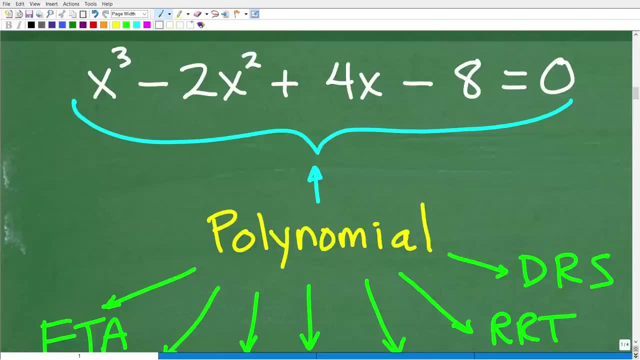 smart in algebra, and that is the goal. so let's go ahead and continue on here. all right now. if we look at our equation, we can see that all the exponents here are positive integers, whole numbers. so we got three. that's good. that's good two here. this is x to the first. 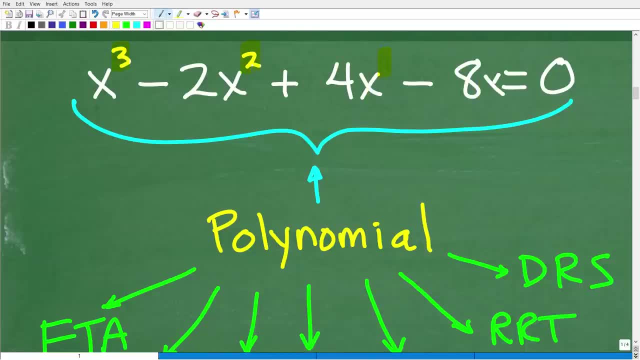 and then here we have a constant, but really you can kind of think of this as x to the zero, anything to the zero. power is one, but that's not necessary. so we have a constant that is a polynomial as well. we can think of it, as you know, being in the polynomial. 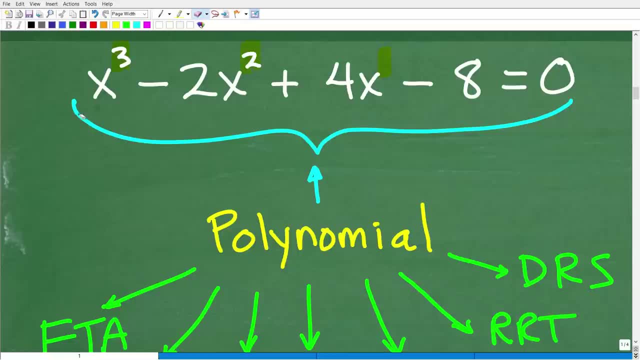 classification, if you will. so we have an equation. all these monomials, these terms are polynomials, so the whole thing is a polynomial. that's really important. again, you know, if you had some sort of rational exponent up here, then what we're going to talk about does not apply. 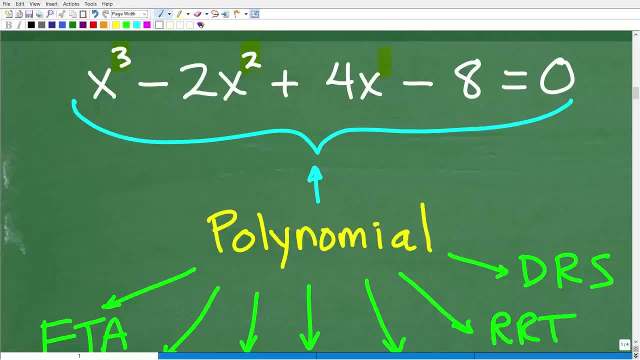 okay. so we love polynomials for multiple reasons, and even in more advanced math-like calculus, polynomials are awesome because we know a lot about them. all right, so we have a third degree polynomial equation. that's the highest power of this equation. so what do we know about solving? 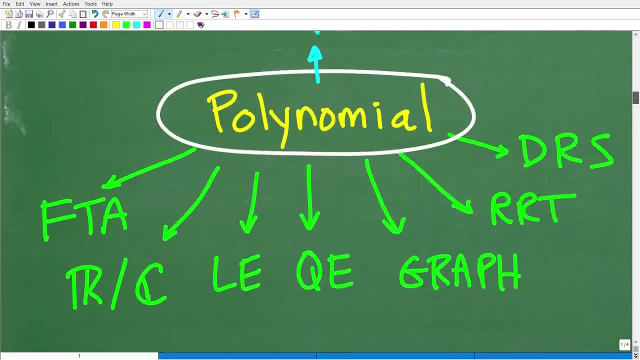 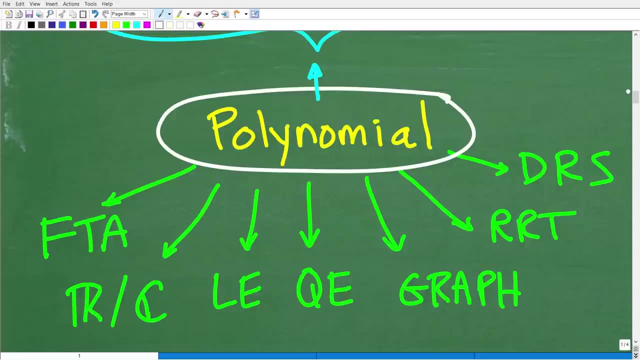 polynomial equations. all right, so I'm going to get into this right now. so here are some things that we can think about, or we need to be thinking about, when we solve a polynomial equation. all right, so the first thing is the fundamental theorem of algebra, FTA. fundamental theorem of: 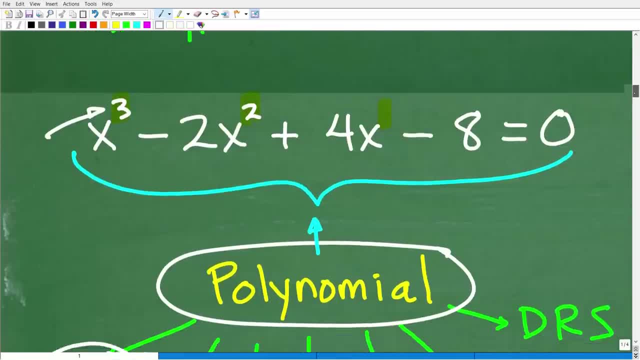 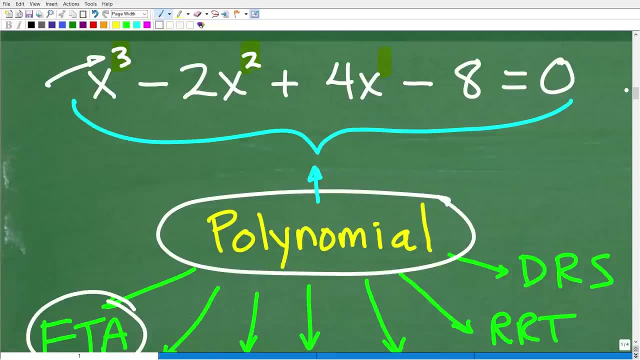 algebra. what does that say Basically? you know the kind of short version of what the fundamental theorem of algebra states is that whatever the highest power of your polynomial equation is, that's how many solutions the polynomial will have. so we have a third degree polynomial equation. so we're going. 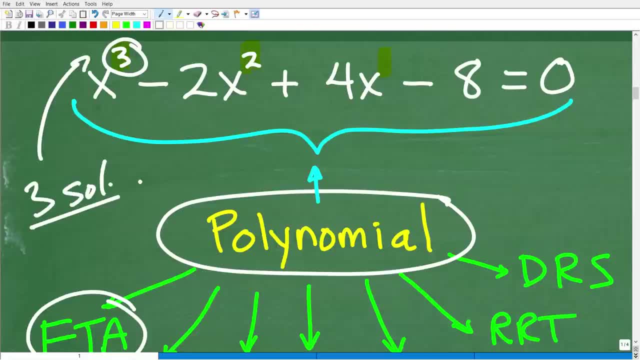 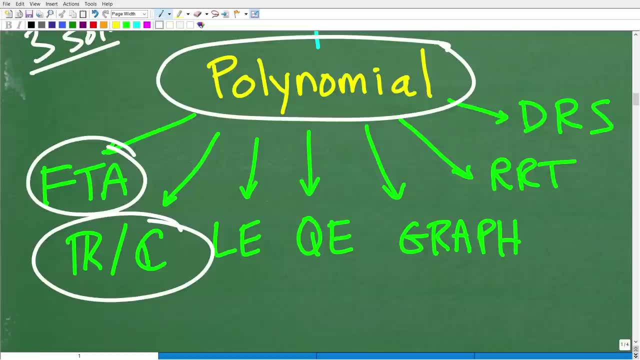 to have three solutions. so that's pretty awesome, because now we know how many solutions we're looking for. but what type of solutions? Well, they could be real. They could be real and or complex, or imaginary, as we have in this case. right, so we have a positive. 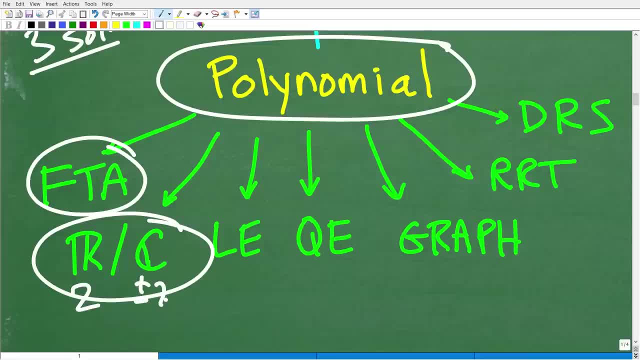 two, that's a real number. but then we have plus or minus 2i, which are imaginary numbers, which are part of the complex number system. okay, now things that you study in basic algebra are like linear equations, you know, kind of like these examples I was giving you at the beginning of 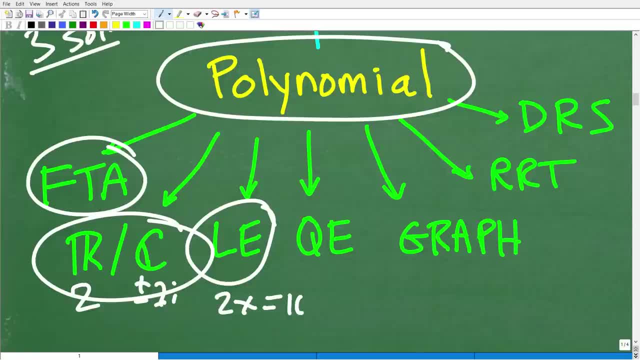 this video, which are just basic equations. 2x is equal to 10,. well, this is a polynomial equation, but we kind of classify this as a linear equation. Then you move on to quadratic equations and you learn a lot about solving quadratic. 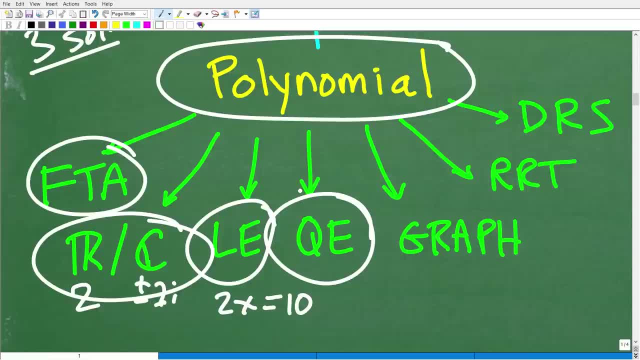 equations to include the quadratic formula completing the square. I mean, this is a huge topic in and of itself. so we're talking about second degree polynomial equations. this has its own, like little world right. so for those of you that have taken first year algebra, 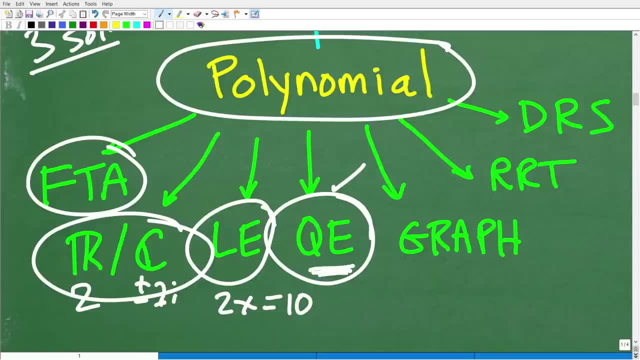 you know that there is quite a bit involved just even with solving quadratic equations. Now, one thing that can really help us is the graph of the polynomial. I gave you the graph of this particular polynomial. It gives us a ton of clues about where the solutions are at. 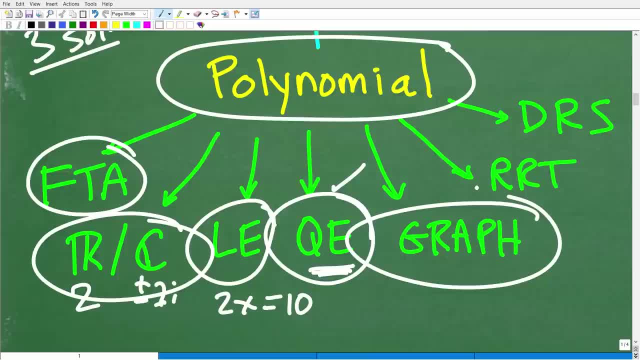 Now, if you have a graphing calculator, you can plug this in and, you know, get some really good hints on where the solutions are at or what type of solutions, And so that's another kind of thing that you could use to help you solve polynomial equations, especially third degree and higher, because it gets much more advanced. 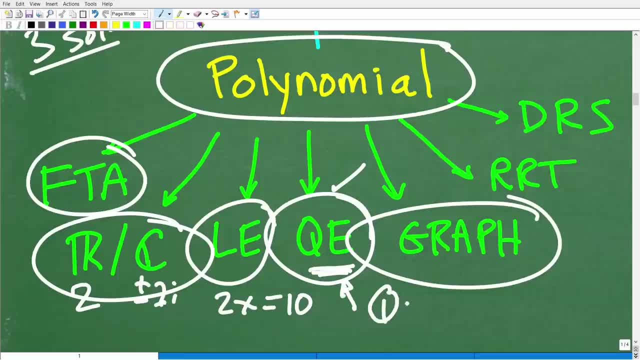 See, in a quadratic equation we have the quadratic formula. Now the quadratic formula will solve any quadratic equation. It's awesome We have a formula that can solve any problem. Third degree: we don't have a quadratic equation type of formula that can solve this. 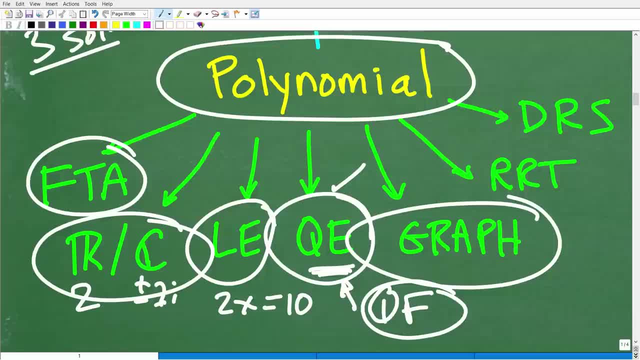 So we're going to have to use all of our knowledge and it gets much more complex. OK, so these last two things are concepts or topics that you study when you get into more advanced algebra, So this is called Rational root theorem. We're going to talk about that later in this video. 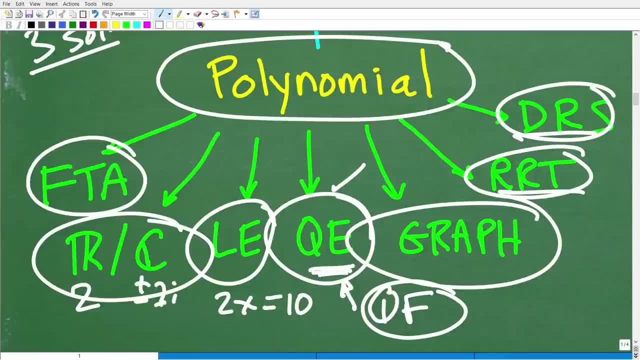 And this other thing is called the Descartes rules of science. So there is a lot, And I'm even leaving some other stuff out. You know, again, this is, you know, a big topic in math And if you're overwhelmed, I'm going to give you some suggestions on how you can really really master this stuff. 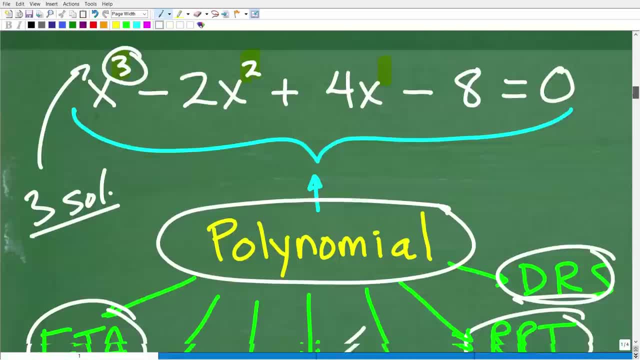 But again we want to frame the problem. We're like: all right, we've got a polynomial equation. I need to be thinking about all these things. So far, we know, hey, we got third. It's a third degree. 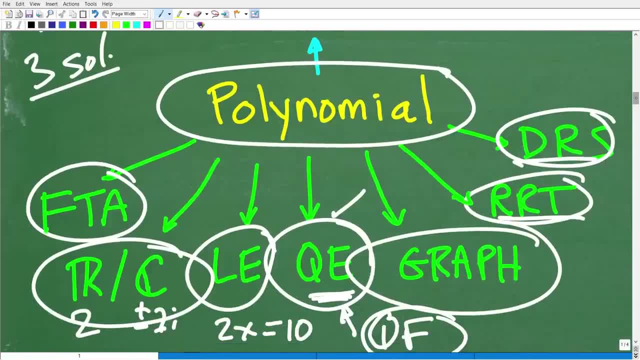 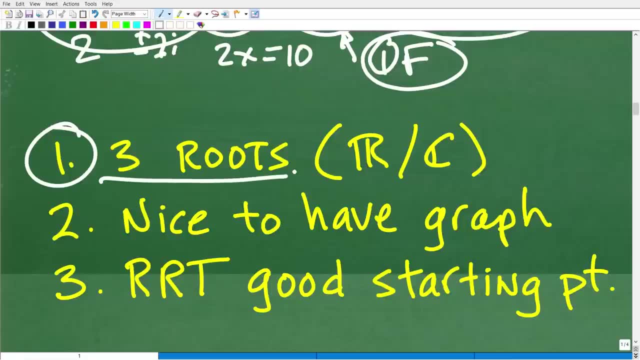 We're going to have three solutions, But we need a strategy to solve this, And that would be this, All right. So, first of all, we know we have three roots. Now sometimes you'll hear the word roots, zeros, solutions. 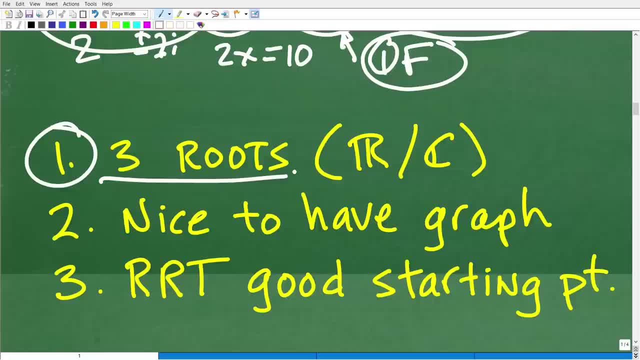 They're pretty much the same, They're synonymous. So the roots Now. there's little technical differences and stuff. But when you hear roots of a polynomial, or zeros or solutions, again these are pretty much the answer to the equations. All right, 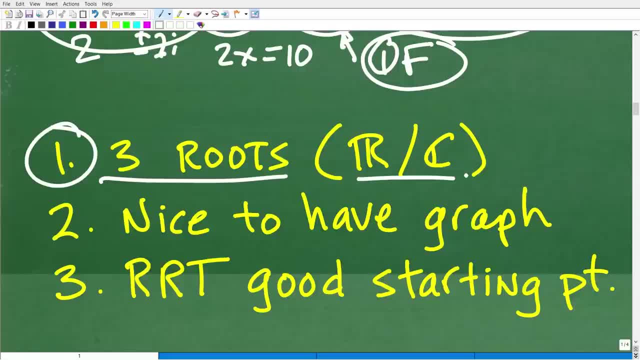 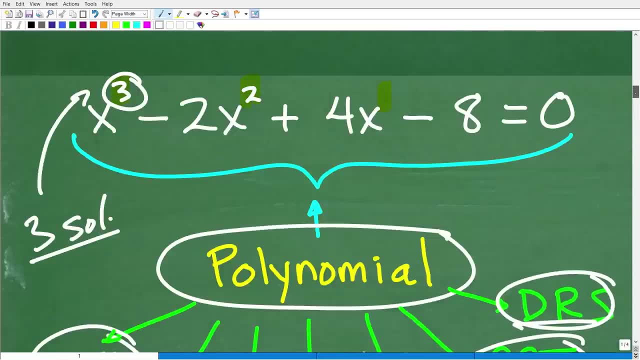 So we have three of them, But we just don't know if they're real Or complex. Now it would be nice to have the graph, And if you're pretty good at graphing, we can literally graph this polynomial. Now that would be a problem in and of itself if we don't have a calculator. 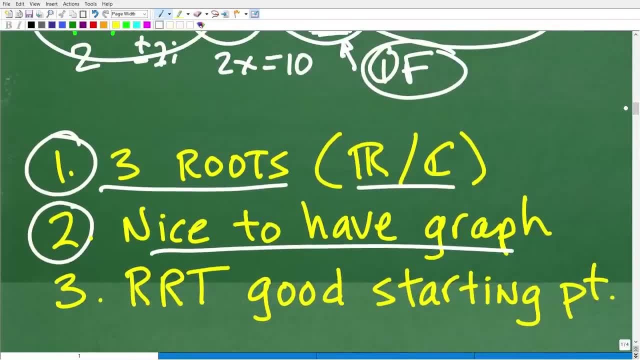 But we could construct it and get an idea of what type of roots and where those roots are at these solutions. But the best thing to do here is to start with the rational root theorem. OK, This is our kind of main starting point. 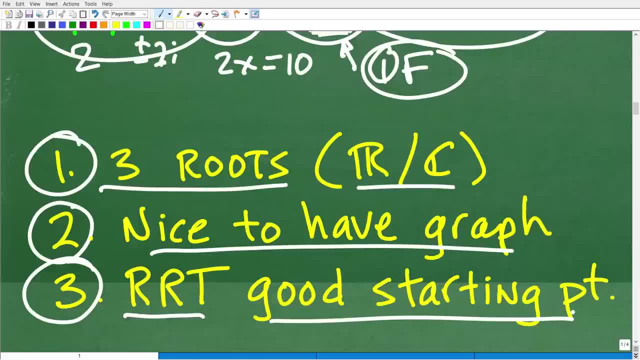 So when you are faced with these type of problems And you know your algebra class or your math class, your teacher is going to want you to start thinking about the rational root theorem. OK, So I'm going to get into this right now. 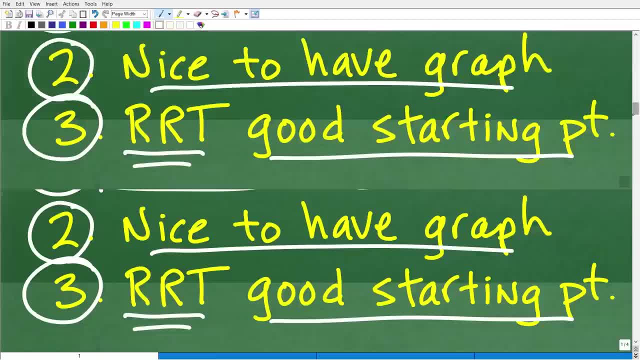 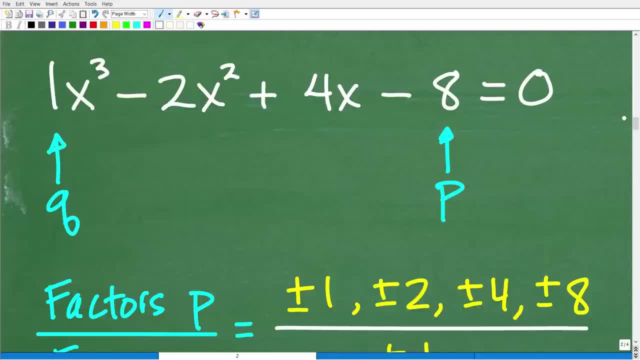 So let's get going to the next step. I know I'm talking about a lot of things, but just imagine how much smarter you're going to be when this video is done. All right, So we are going to get into the rational root theorem. 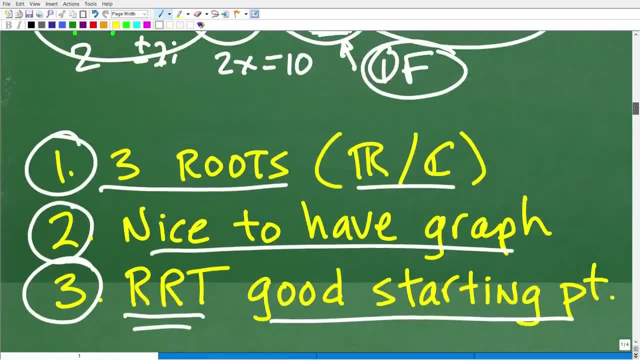 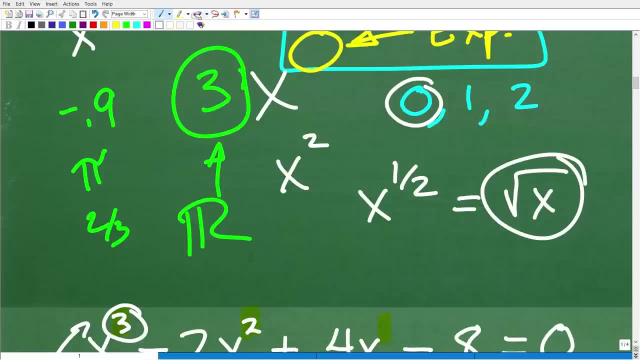 Now, before I even start, OK, What is the rational root theorem? All right, Now a rational Rational root. OK, Let me go back over here. So I really want to, really want you to understand this concept, All right, 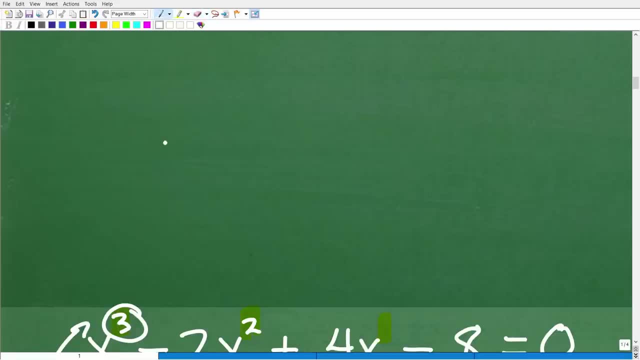 So we have to go back to what is a rational number. OK, So on a real number line, here's zero, Here's one, Here's two, Here's three, And any number that is like one half, any number that we can express as a fraction of integers is a rational number. 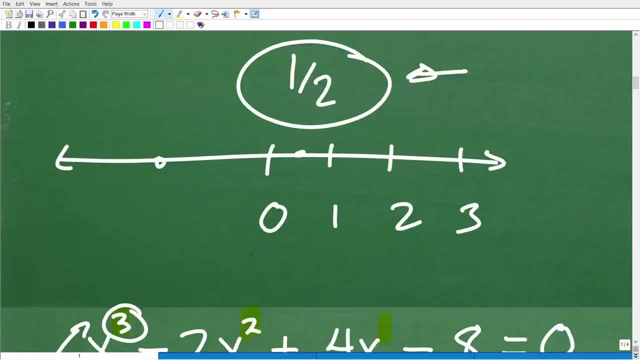 So, for example, One half is a rational number. Negative three halves is a rational number. Two is a rational number because we can express two as two over one. Now remember: a rational number is where the numerator and denominator are integers. 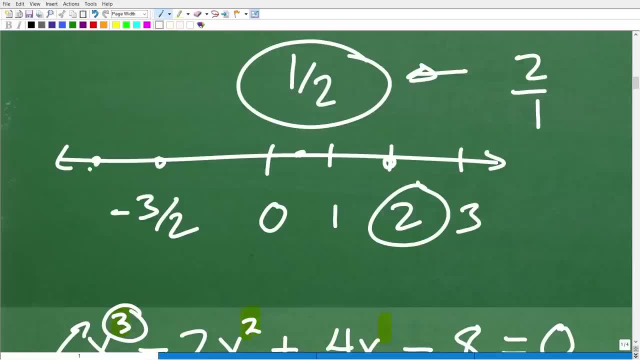 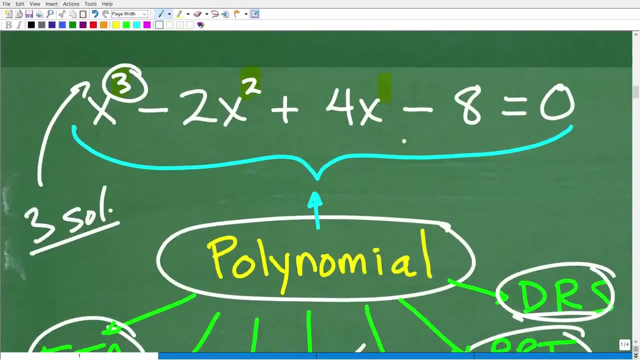 OK, So we're talking about positive negative fractions and positive negative numbers like over here, negative five or three. These were all fall under the classification of rational numbers, So these Type of numbers came when we're looking for the solutions to this equation. 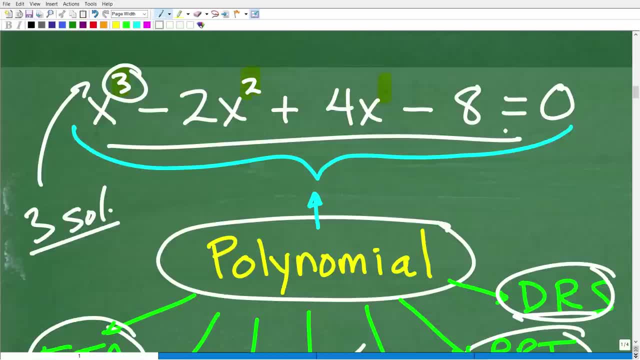 This solution may have rational roots, In other words rational answers. In other words, maybe one of the solutions here is two- Of course, we already know that's the case- But maybe another one is like one half and maybe another one is negative three halves. 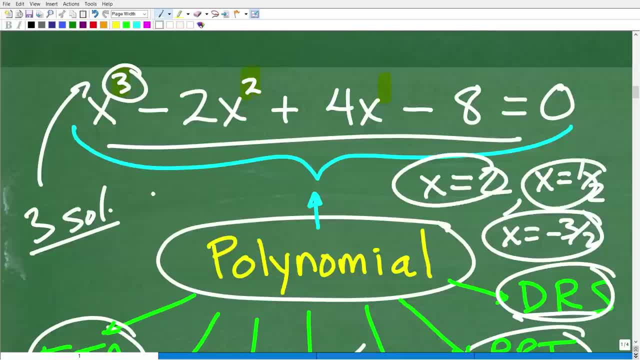 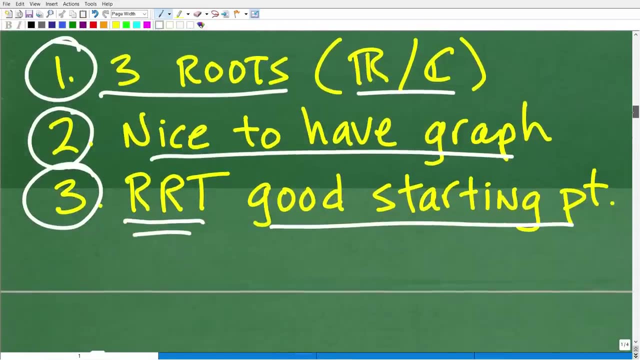 These are rational roots, But you can have other type of solutions here. You can have like: X is equal to the square root of seven, OK, Or positive negative seven. This is not a rational root, but it could be a solution. So the rational root theorem is a way for us to list out all the possible rational roots that this equation may have. 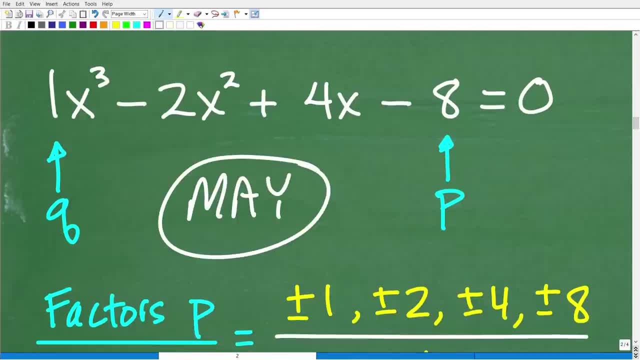 May I have to kind of stress: this may have All right. We don't know if it has rational roots, but if it does, it's going to be part of this list that we're going to construct. OK, So let's go and get into this right now. 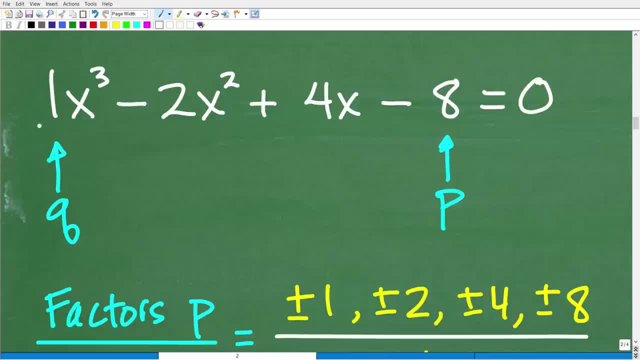 So what we need to do first is list our Polynomial from highest to lowest power, So third degree to eight. This is what we call standard form. Now, the leading coefficient- here we're going to label that as Q, And then our number over- here we're going to label that as P. 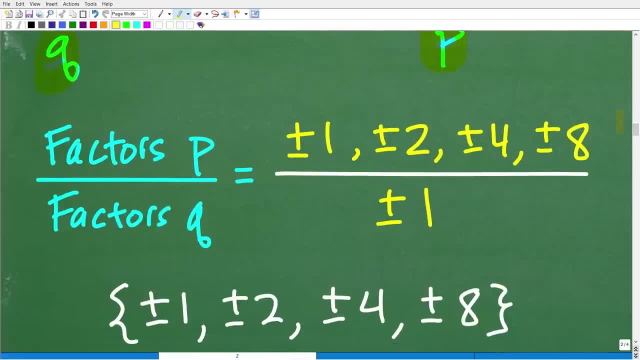 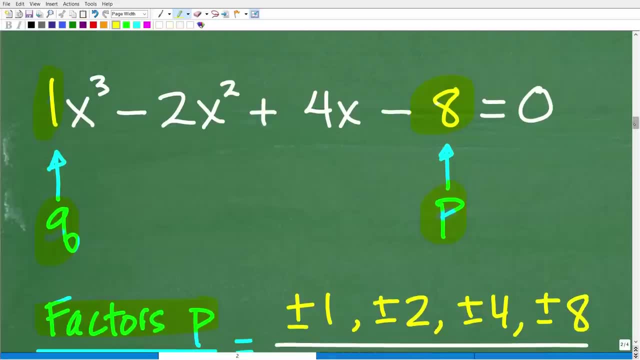 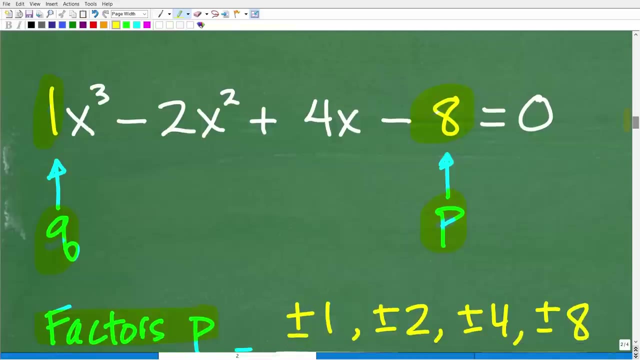 OK. So here is the rational root theorem. So it basically says the factors of P. OK, Which is the constant value right over here. In this case it's negative eight over the factors of Q And this particular problem, the factors of Q, is one right. 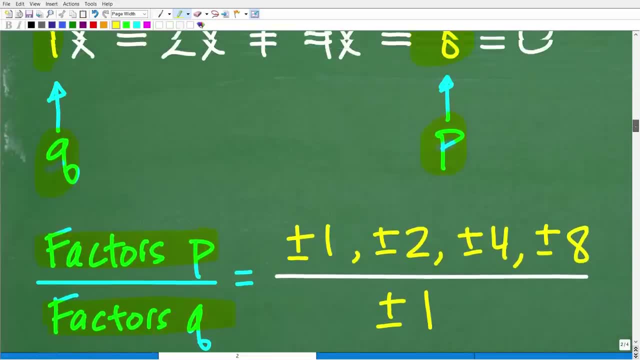 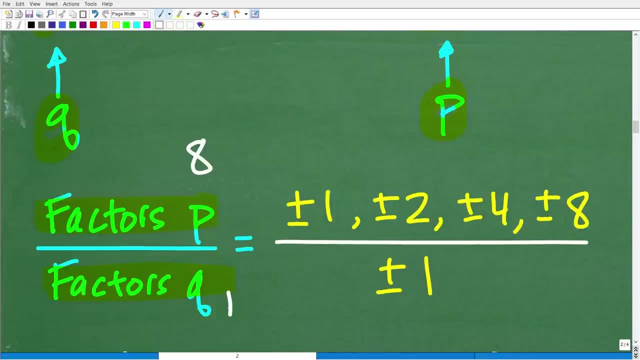 So that's one. So we're going to list all the factors of P and Q. I'm going to create a fraction. This is a fraction, right? So the factors of P over the factors of Q. So this is eight and this is one. 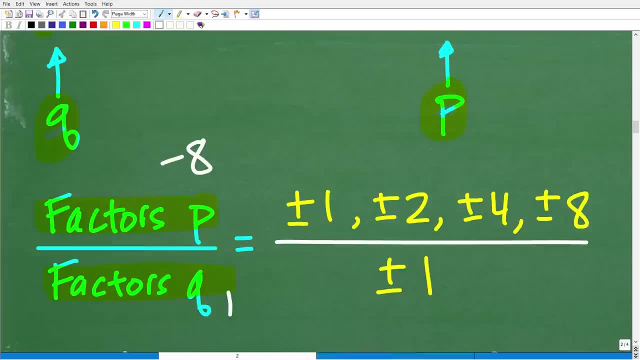 Doesn't make a difference if it's negative or positive, We're going to still have the same factors, OK. So what are factors of eight? Well, positive and negative one. OK, Because negative one and times negative eight can get us to a negative one times. 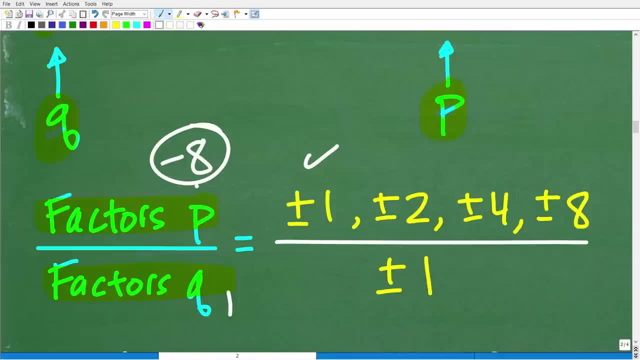 Negative Eight gets us to a positive eight or negative. one times a positive It gets to a negative. So just what you want to do, It's always going to be positive and negative, right? I'm kind of speeding up here, because explaining the rational root theorem is like a full lesson in and of itself. 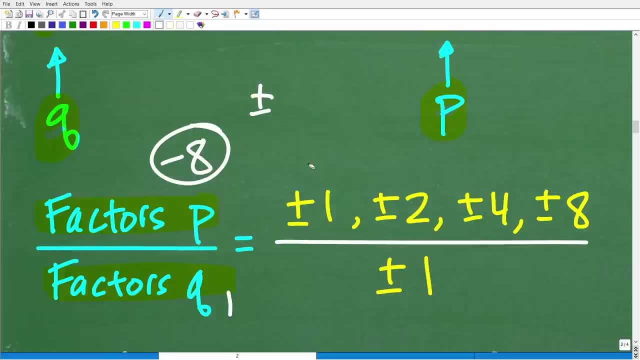 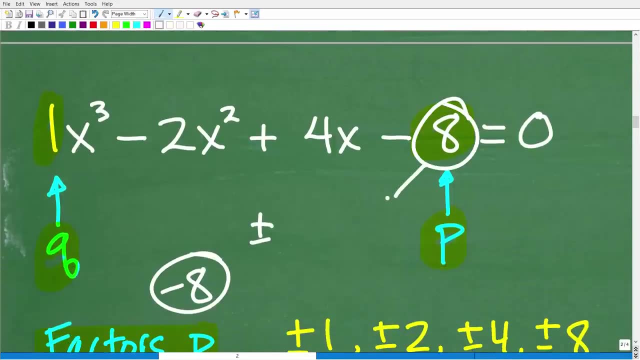 So we're going to pick up the pace here, All right, So, so again, whatever this number is, you're going to just start listing out the factors of eight. So you're like, all right, well, one is a factor of eight. 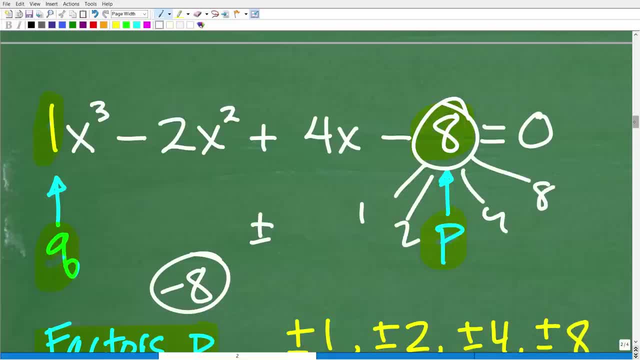 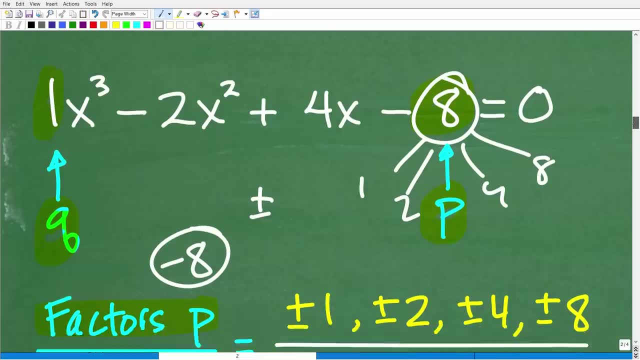 Two is a factor of eight, Four is a factor of eight and eight is a factor of eight. So we're going to list them, One with positive and negatives, just like this. OK, Now, factors of one. Pretty easy, That is just one. 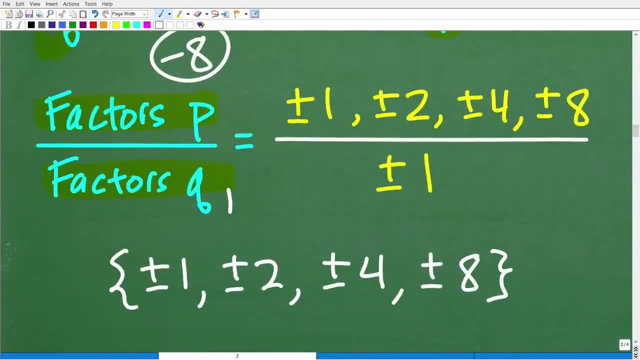 So positive, Negative one, All right. So this is a fraction. Now what we're going to do is take every possible iteration of the numerator and denominator. So one divided by one positive, negative, one divided by positive, negative, one is what? Well, that's going to be a one, right one divided by one, two divided by this one is: 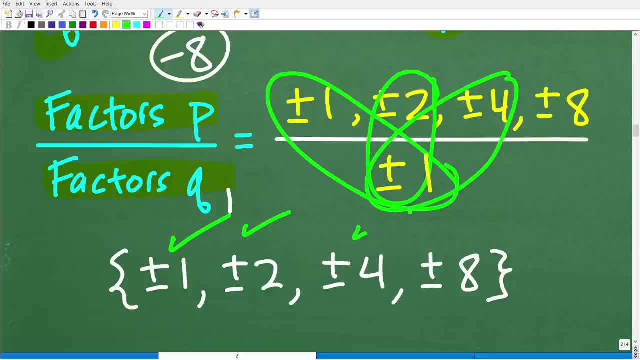 two positive, negative. Four divided by one is going to be four, and eight divided by one is going to be eight. All right, So no problem there. Now here. OK, You can see we have a list, OK, So we just kind of basically divided this denominator by all of these possible numerators. 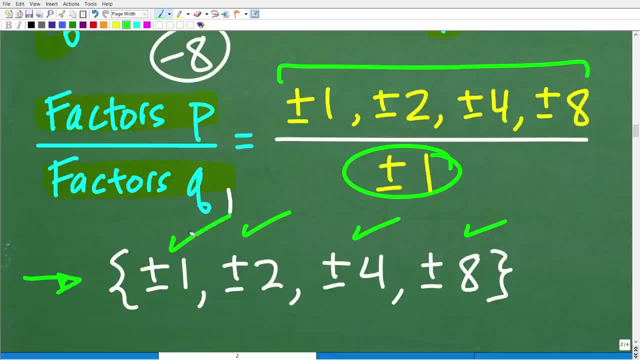 Now we have this lovely list. This is what we worked so hard for, And this list is the possible route of rational roots. OK, Let me say this in a different way. If our equation here has a rational root, or rational roots, it will be among these numbers. 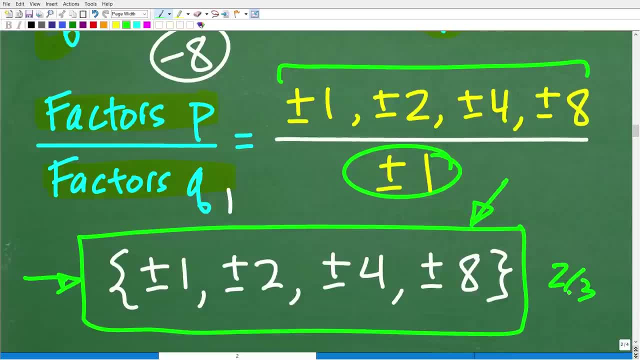 right here. In other words, we're not going to have like two, thirds or five because that's not on this list. So here we have possible solutions, at least one or maybe two or maybe all of them amongst this list. So we need to start testing these possible rational roots. 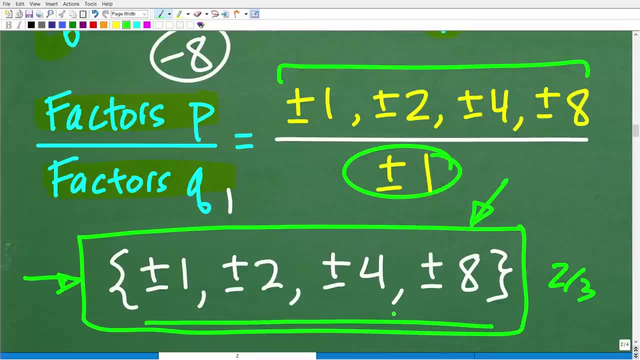 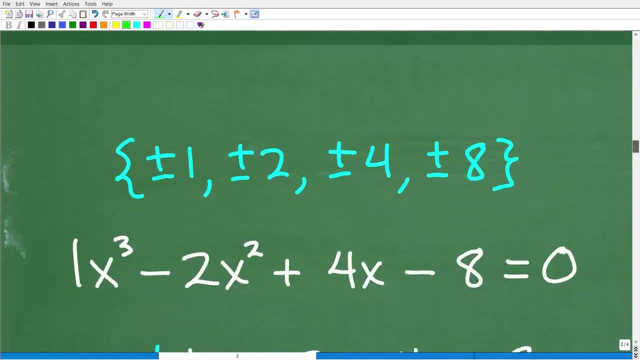 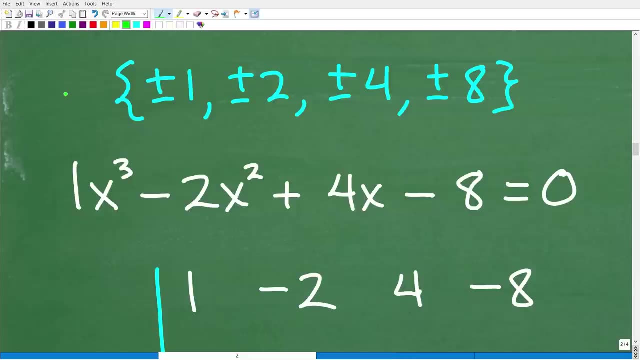 And the hope that we actually have a rational root, because that's going to allow us to solve the rest of the equation. All right. So let's go ahead and start doing that right now. So here is our list, And this is going to bring us to another lovely topic called synthetic division. 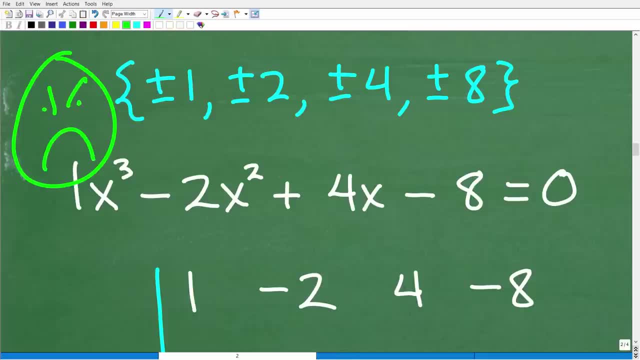 Now I know a lot of you at this point are like Mr YouTube: Math Man, I'm done, I quit. My hair is just on my ears. I got smoke coming out here. Well, listen, take it easy, Take it easy. 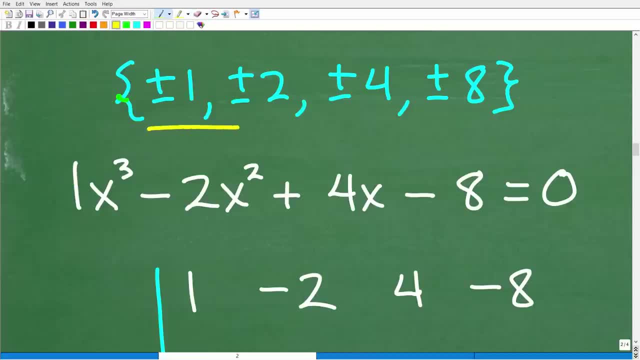 We're going to do this one step at a time, But what we want to do is test these solutions to see if, in fact, they are good. Now you could plug them in as I described. we can take this one and plug them in, right? 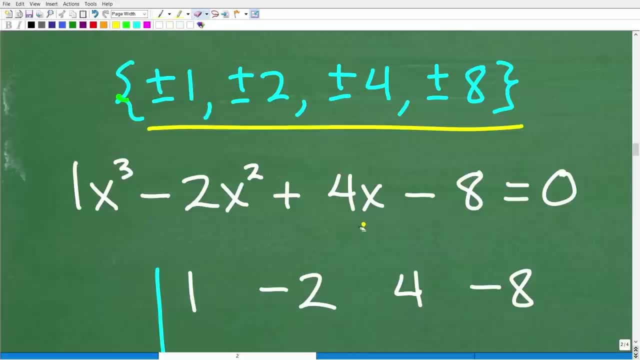 here, But that is not the most efficient way to do this testing. Okay, What we want to do is: do we want to do something called synthetic division, And this is another big topic that involves a polynomial long division. Okay, It's kind of a shortcut. 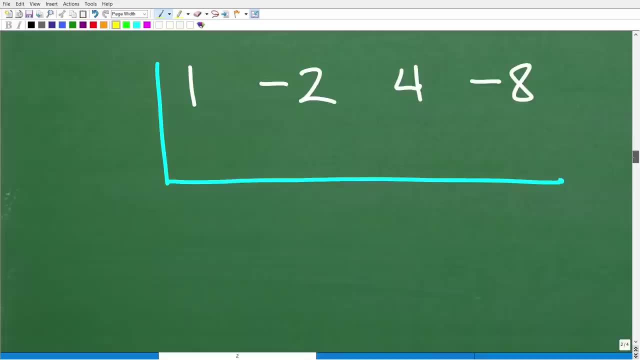 So I'm going to show you this. This is going to be pretty cool here, And hopefully most of you watching this video have studied this before, so you kind of know what I'm doing. All right, So here is our polynomial. Now notice. we have the coefficients here: 1, negative 2,, 4, and negative 8.. 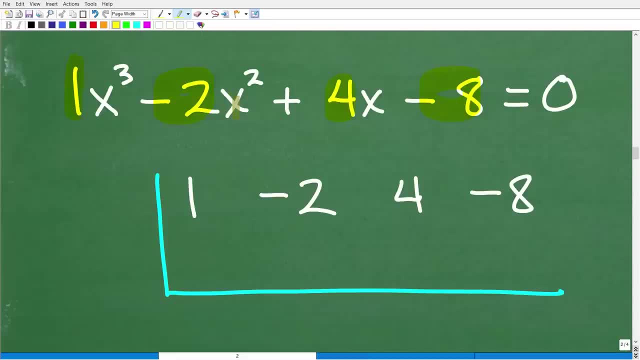 Our polynomial must be written in standard form and all terms must be represented. In other words, we can't go from X cubed to X. We need to. if we were missing an X squared, we'd just put in a zero X squared. 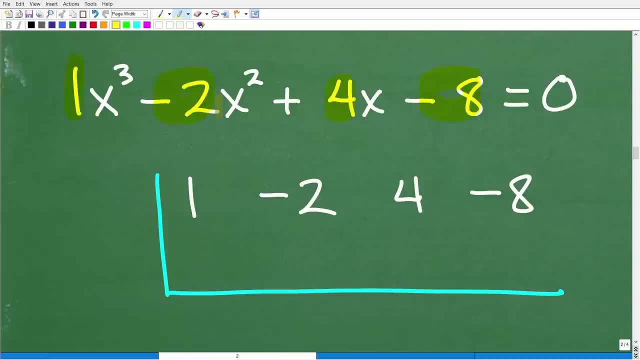 Okay, All right. So again, I'm covering a lot of territory. So what we're going to do is write these coefficients just like this: 1, negative, 2, 4, negative, 8.. Right, So they're coming from these coefficients, right here? 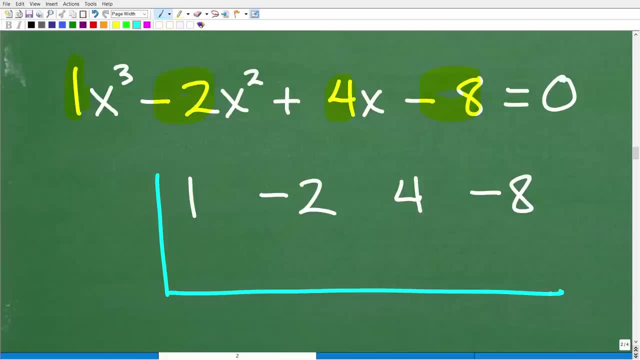 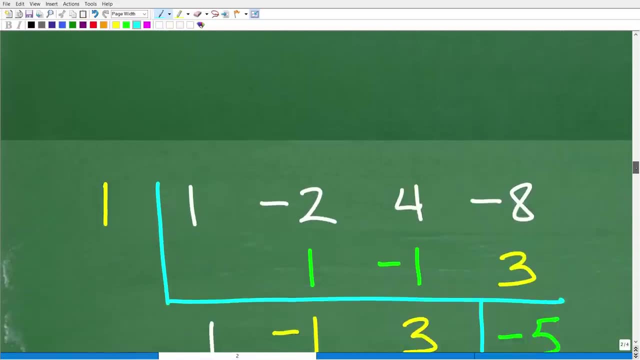 And then we're going to draw this lovely kind of L bracket like. so All right, So this is the setup for synthetic division, All right? So now let's go ahead and start testing some of these solutions. Now let's start right here. 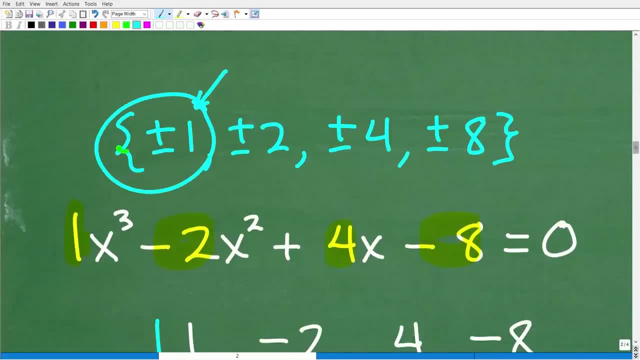 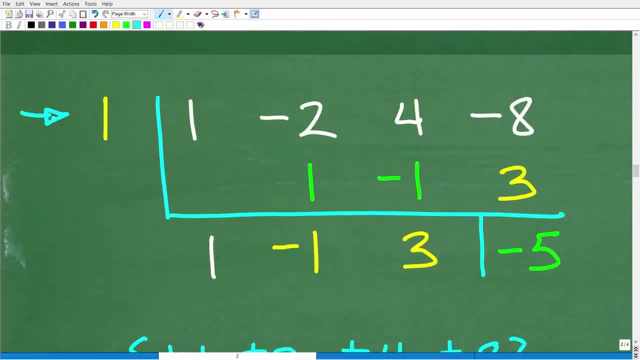 We have positive and negative 1.. Let's test to see if 1 is a solution. So this is how it works. So we're testing 1 and I'm going to show you the process right now. Okay, So what we're going to do is take this first number in this setup and we're going to drop. 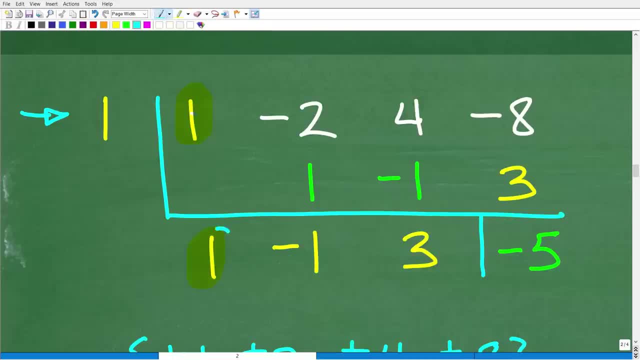 it down here. In this case it's 1.. Okay, So we're going to take this 1 and we're going to drop it down here. Okay So, whatever this number is, you're going to write it right down here. 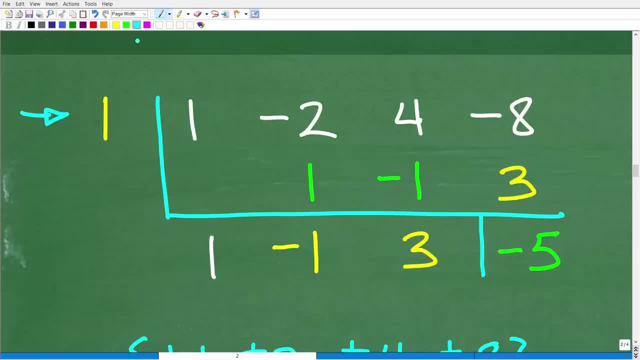 Now I already did the problem, but I'll repeat this in a second And in real time, so you'll see. So you're going to take 1 times this, 1.. Okay, 1 times 1 is what? 1.. 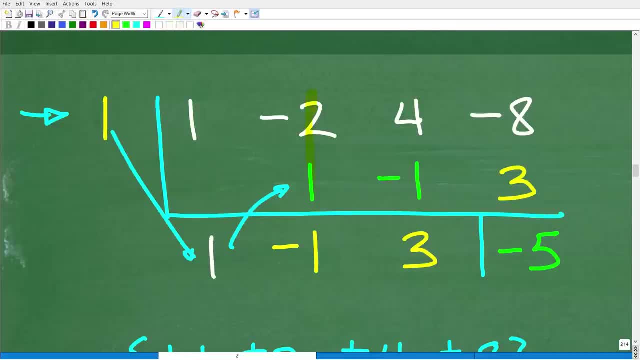 You put your answer right there. Okay, Now you're going to add down: Negative 2 plus 1. is what Negative 1.. Negative 2 plus this, positive 1, negative 1.. Now we're going to repeat the process. 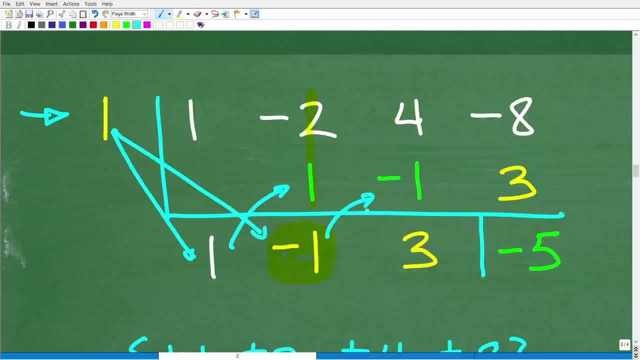 1 times negative: 1 is what Negative, 1. Now we're going to add down 4 plus negative: 1 is a positive 3. Now we're going to repeat the process: 1 times 3 is 4.. 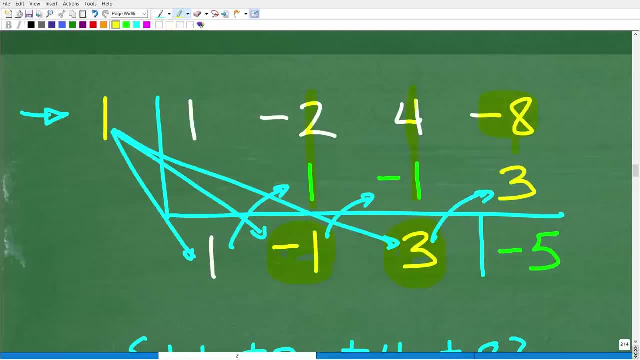 Plus 3 is 3.. And then we're going to add down Negative 8 plus 3 is negative 5.. This is what we call the remainder. Okay, Now notice we have negative 5 here, right? Well, that tells us that 1 is not a solution. 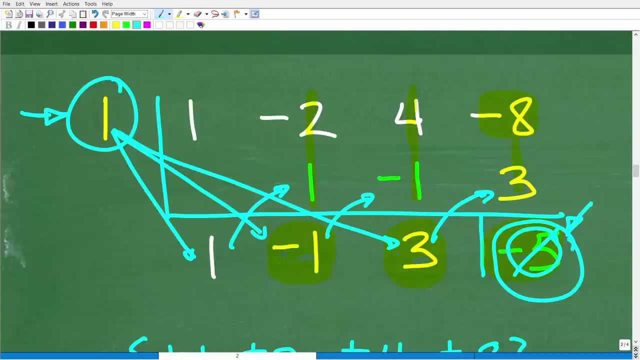 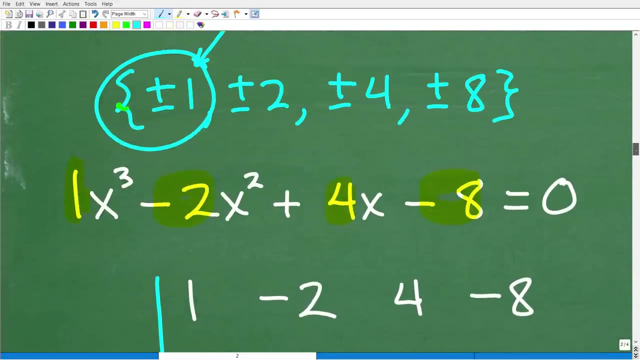 What we're looking for is our remainder to be 0. If our remainder is 0,, then this number is a root. It is a solution. So we're going to use synthetic division to test these values. Okay, So what you would do is you just start going through your list here. 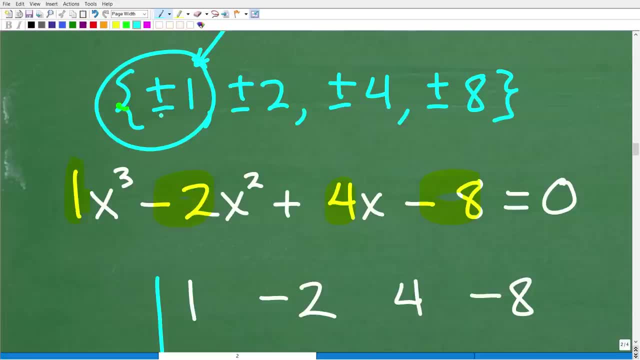 So we'll test 1 and negative 1.. I'm not going to test negative 1 because that's not a solution, But 2 is a solution, right, because I already told you the answer, So let's see how that works. 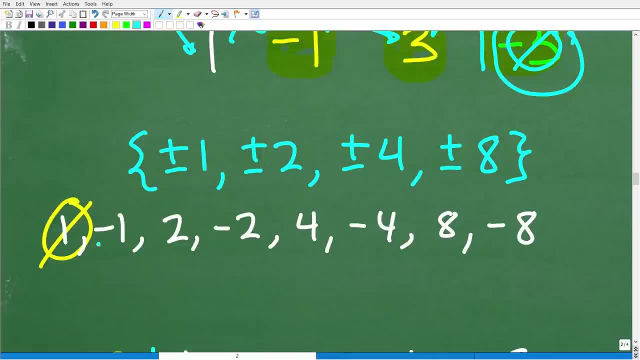 All right. So we go through our list and we're like, all right, 1 is not a good solution, So we move on to negative 1.. Then we try 2.. We move on to negative 2.. It's a lot of work. 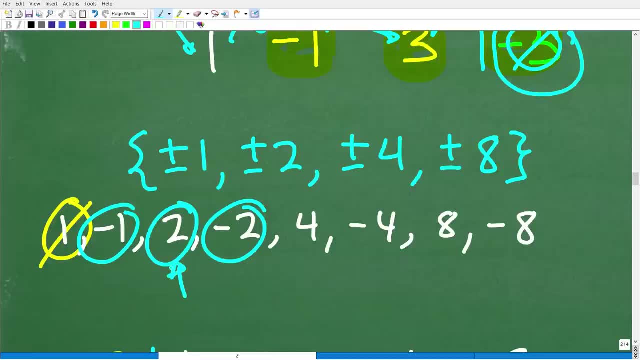 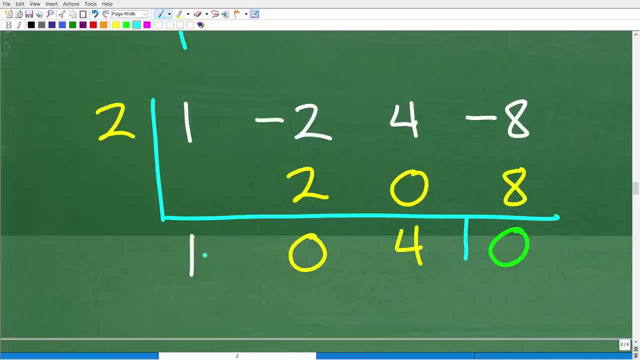 Yes, I know it is, But anyways, let's go ahead and continue on And let's test 2, because we know that does work. So let's see how this plays out. Okay, So here's 1.. We're going to drop it down, just as I indicated. 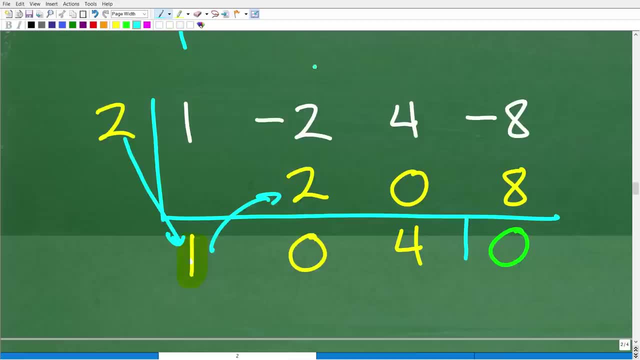 And now we're going to start the process. 2 times 1 is what? 2.. Okay, We're going to add down Negative. 2 plus 2 is 0.. All right, So 2 times 0 now is 0.. 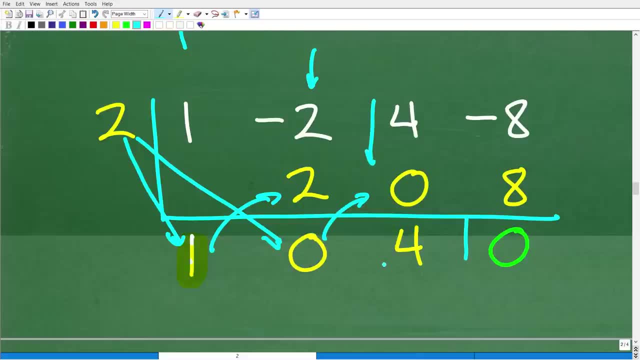 Okay, And we're going to add down: 4 plus 0 is 4. And then 2 times 4 is 8.. Negative: 8 plus 8 is 0.. All right, Awesome, 2 is a solution. 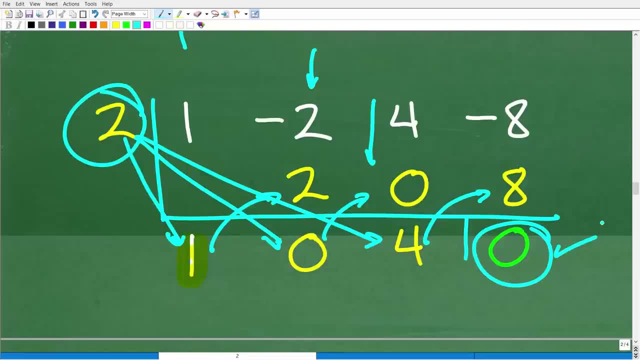 Mm-hmm. Okay, Because 0 is a remainder. Now we can take the next step to figure out the rest of the solutions to this polynomial equation. All right, But let's go ahead and take the next step right now, and that is to quickly subscribe. 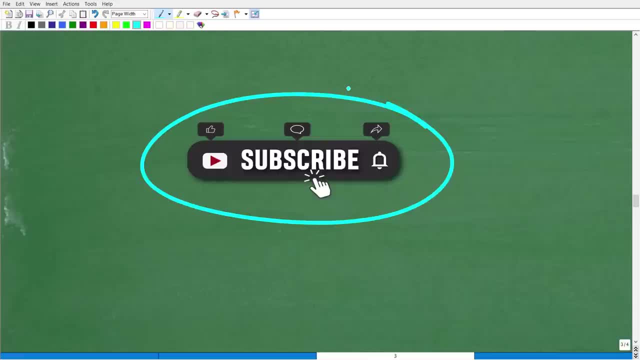 to my YouTube channel. You usually kind of babble on for like a minute on why you should subscribe, but we have a lot more work to do here, So I'm just going to tell you quickly: subscribe. It's really important. You can see, this is a ton of work to put together and teach this stuff. 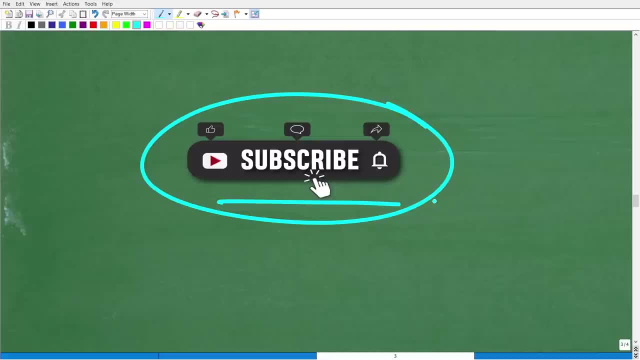 I love teaching mathematics, but I need your support to be able to kind of continue on. But, most importantly, I need your support so I can reach as many people as possible, Because imagine someone who doesn't really understand this. They're going to be like: I don't get this. 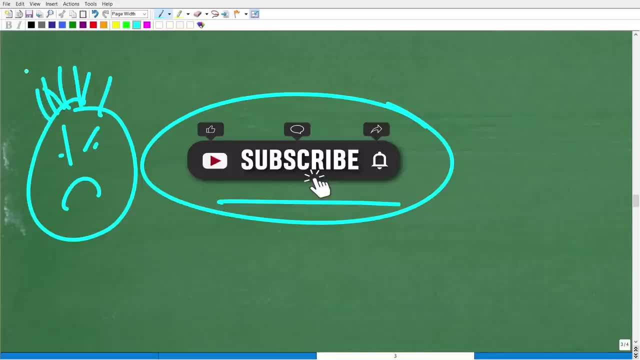 I quit math. I don't want to study it anymore. Well, I'm trying to really break these concepts down in a clear and understandable way Now, before we get going. okay, for those of you that really need to understand this level of math, I got two recommendations. 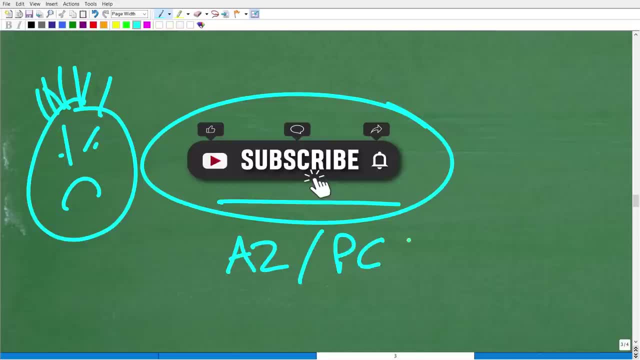 I got two recommendations for you. Check out my Algebra 2 and or Pre-Calculus course. I'm going to actually strongly recommend my Pre-Calculus course to master everything that we're talking about. You'll find links to those in the description below. 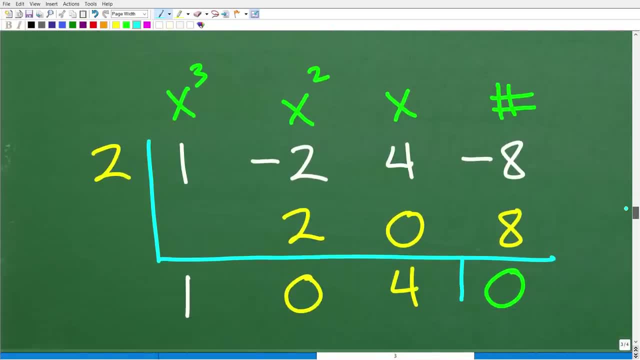 All right, so let's go ahead and continue on here. So we test, we tested two and we have the remainder zero. So two is good. Now what does that mean? Well, here remember: one was the coefficient for x, cubed. 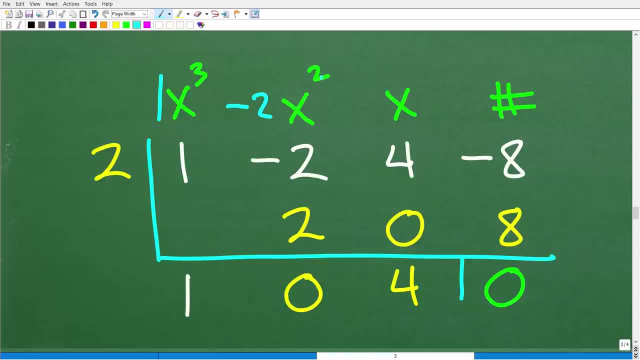 The negative two was the coefficient for x squared, and then we have plus 4x and then minus 8, right. So that was our equation. Now, this is the way it works when you're doing synthetic division. These right here: this one is our x cubed, this is our x squared, this is our x and this: 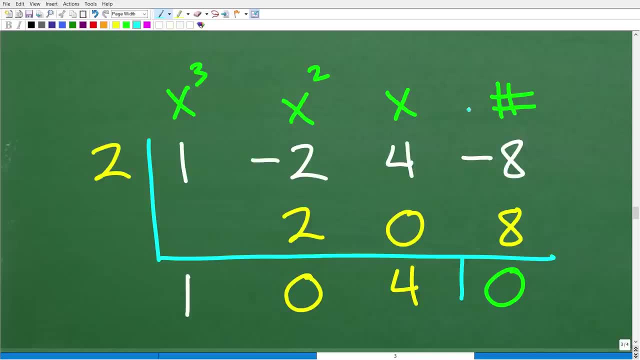 is our 8.. These numbers are on that, you know. these are the respective degrees. Now our answer down here drops down one degree. So if this is x cubed, our answer down here is x squared. okay, And so instead of an x, this is now a number. 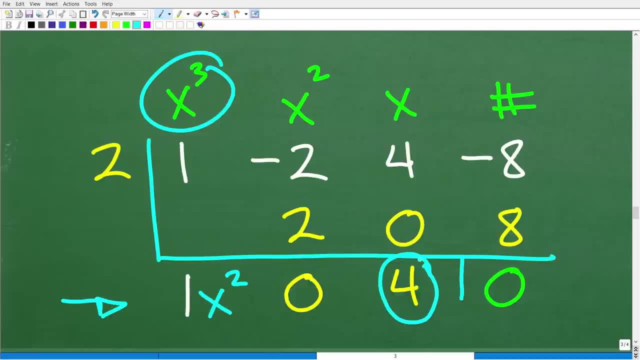 I know this is confusing because I'm trying to cover a lot of territory quickly, but we know that x is equal to 2 is a solution, So now what we have is 1x squared plus 4 as a remaining linear factor. okay, 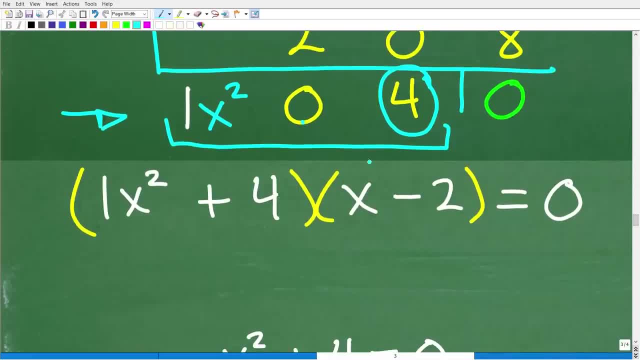 So, in other words, we can literally write this as 1x squared plus 4 times x minus 2, because you know this is a linear factor, Because we know that 2 is a solution right, And if we set this equal to 0, remember, this whole equation is equal to 0, we got x is. 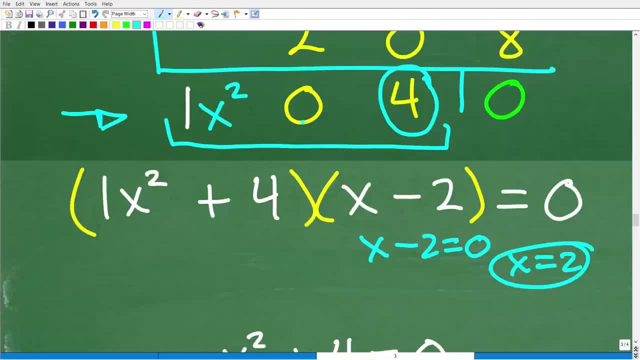 equal to 2, okay, So that's pretty awesome. So this is the other linear factor. So now we have 1x squared plus 4, and now we just need to solve this to find our other two solutions. Remember, we have three solutions here. 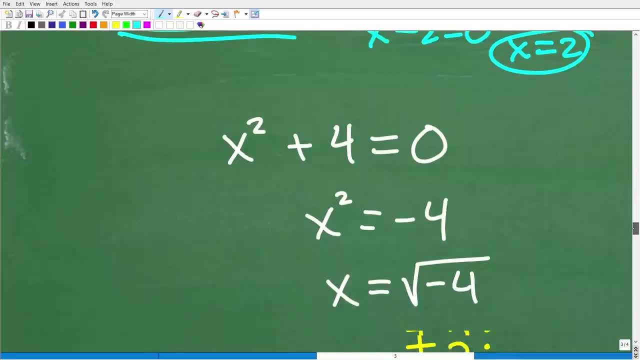 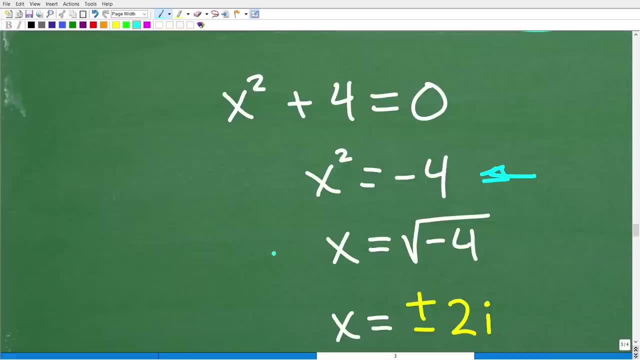 All right. so we're going to set x squared plus 4 equal to 0 and solve. So we're going to subtract 4 from both sides of the equation, we get x squared is equal to negative 4.. So we're going to solve this lovely quadratic equation by taking the square root of both. 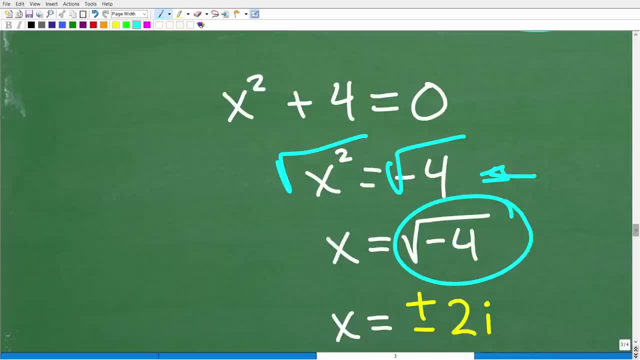 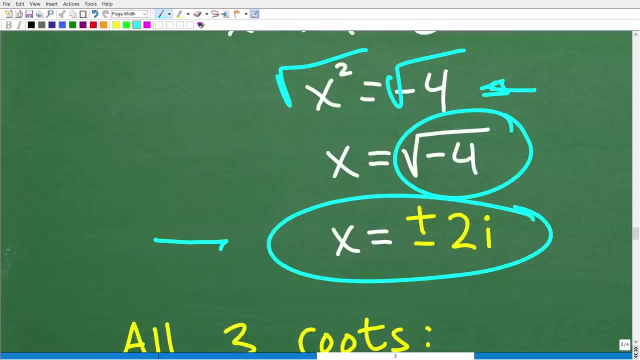 sides, And when we do that, we're going to take the square root of negative 4, which, of course, is an imaginary number. That's going to be equal to positive negative 2i. Hopefully you understand what's going on here. 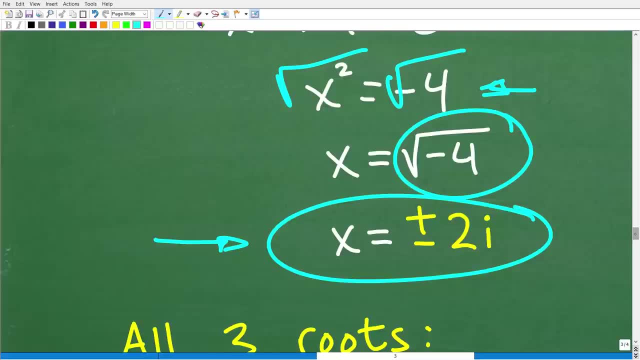 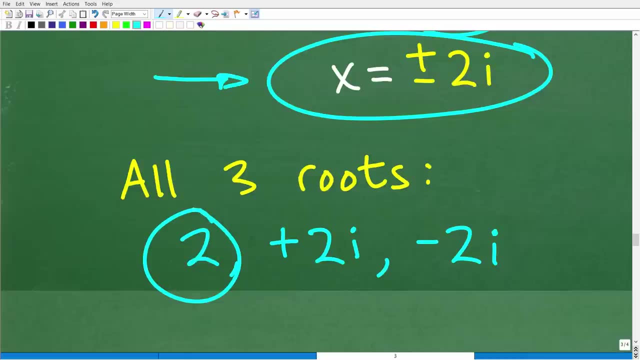 And again, these are two unique solutions, okay. So our three specific solutions is 2,, okay, which is a real number, rational root, and then we have positive Now, positive 2i and negative 2i. here's our three solutions per the Fundamental Theorem. 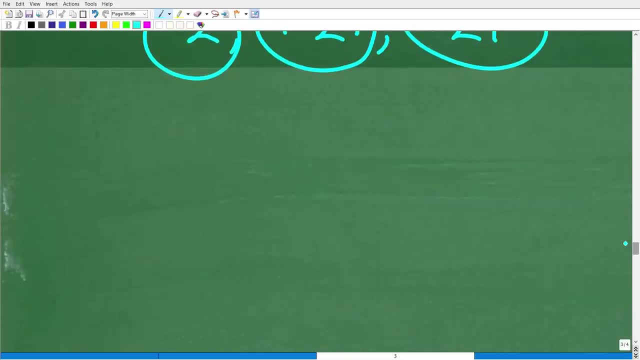 of Algebra, And I know some of you are exacerbated by this. You're just like Mr YouTube Math Man boy. well, you know, maybe you're saying this. Thank you so much, I finally get it okay. Well, I hope that's the case. 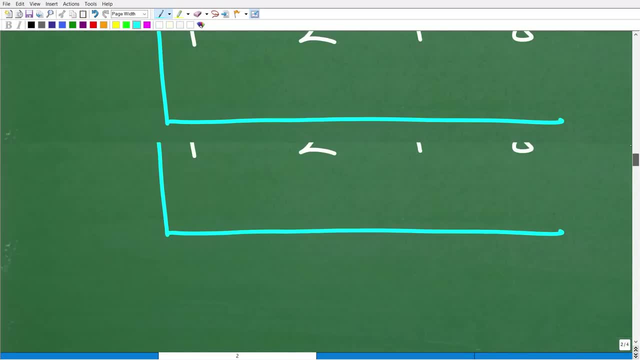 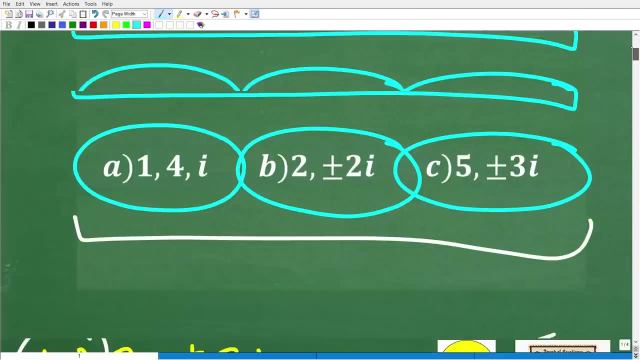 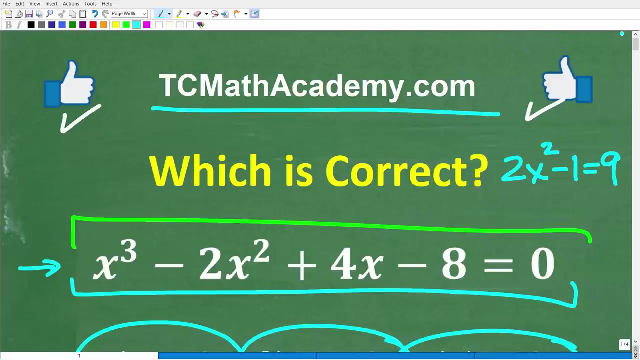 I covered a lot of material- okay, Pretty much did multiple chapters of algebra in this one video, but sometimes it's good to kind of see the summary of where things go. But this is stuff that you need to know at this level of math. all right, 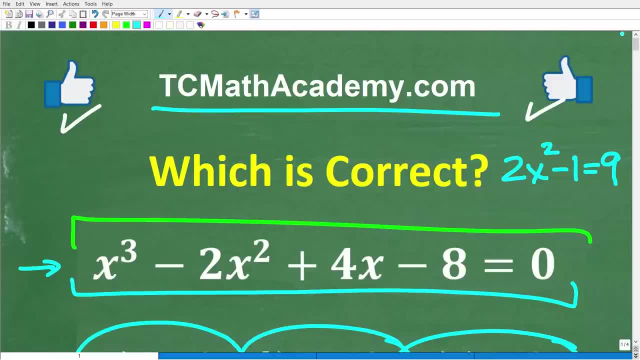 Unfortunately, there's no way of getting around it, but if you need help in this, okay, make sure you get it, either from myself or from someone else, because it's only going to get more challenging again if you plan on continuing on in math, and I hope you do-